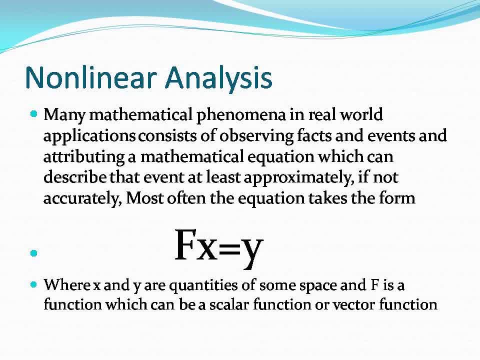 So this is the most general form of the equation fx equal to y. These type of equations can be linear or non-linear, depending on as whether f is linear or non-linear. If s is linear, we call this equation as a linear equation. If f is non-linear, we call this equation as a non-linear equation. 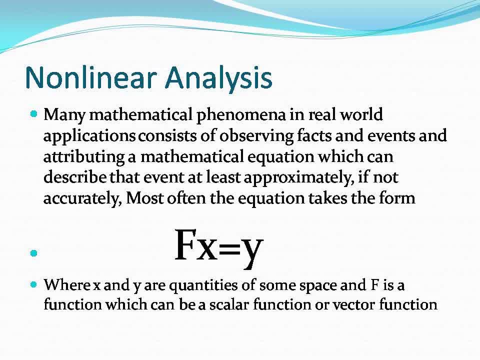 And there are various techniques and various theory how to solve this equation. For example, if you have some matrix, then we can just take the inverse of the matrix, where x equal to f, inverse of y, and we can solve the equation. But in other cases there are various other theories which lead to the study of solving such equations, and one such technique is called the fixed point technique. 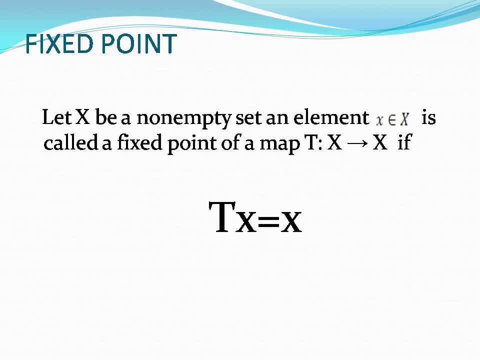 So in a fixed point technique we have a non-empty set, x, capital X and an element x is a non-empty set, So x belongs to x is called a fixed set point of this map t from x to x. if tx equal to x. 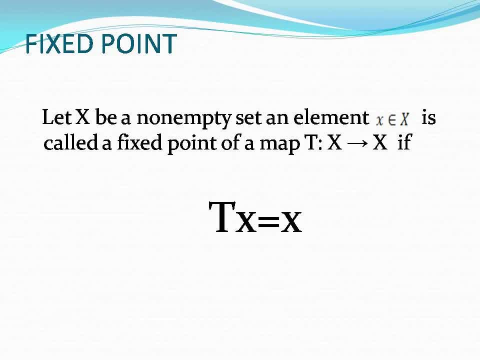 So x is a some space. Normally x contains a space of continuous functions because while solving equations we normally look for a solution in the form of a continuous function. Therefore this x can be a set similar to a continuous function from a closed central, a comma b, or a continuous function from a closed central, a comma b, or a continuous function from a closed central, a comma b. 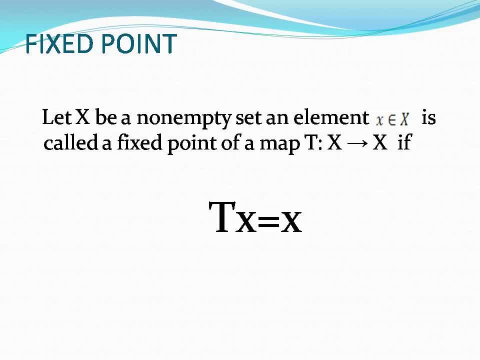 So this is a set of continuous functions. So we call element x. belong to x is a fixed set point. if tx equal to x, A map can have one fixed set point or several fixed set point. There are several theorems which guarantee the existence of fixed set point theorem. 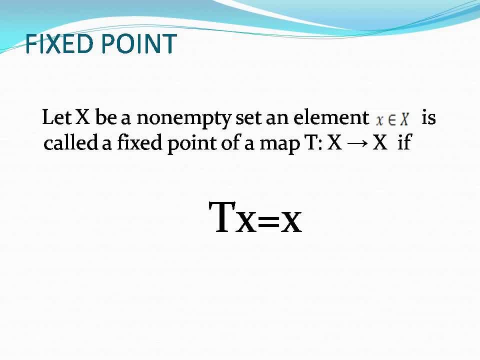 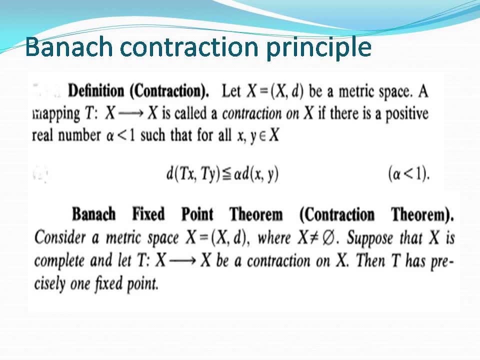 But the most important and the most significant among them is the Banach contraction principle. A banach contraction principle is a non-empty set. x capital x principle is set in the setting of a metric space. A metric space is a set where we have 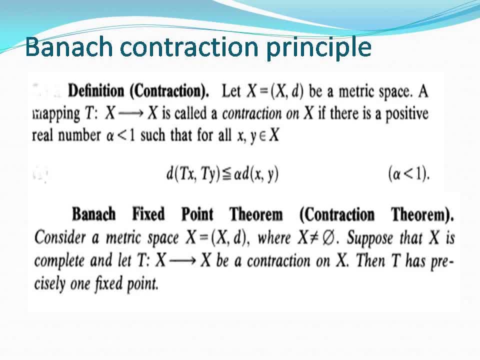 a metric structure. A metric structure helps us to define the distance between any two elements in the set. So if x is a metric space, a mapping t from x to x is called a contraction map. If there is a positive real number, alpha less than 1, such that for all x, y and x 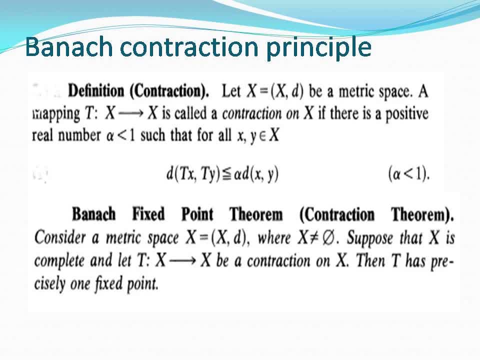 d of tx, ty is less than equal to alpha into d of x- y, That is, the distance between tx and ty is less than or equal to alpha. If alpha is less than 1, alpha times d of x- y is a contraction. We call this a contraction map because the distance between tx and ty. 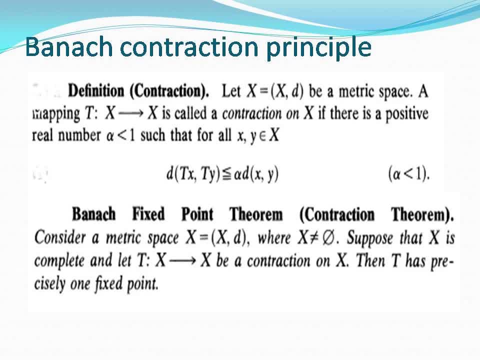 is less than the distance between x and y, So the distance is contraction. So we call it as a contraction, And Bernak's fixed point theorem states that if x is a complete metric space, then any contraction from x to x has precisely one fixed point. 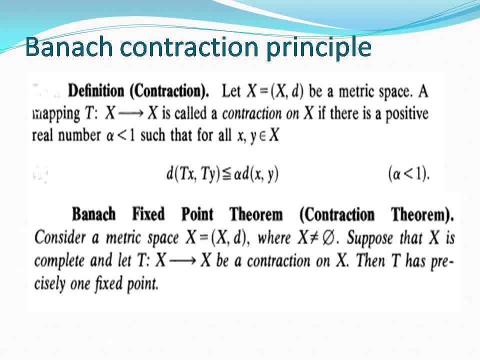 So in a complete metric space, complete metric space means every Cauchy sequence convergence. so every closed subset of a complete metric space is also a complete metric space. So complete metric space, This contains all the limit points. So if t is a contraction on the complete metric space x, then we have the Bernak contraction. 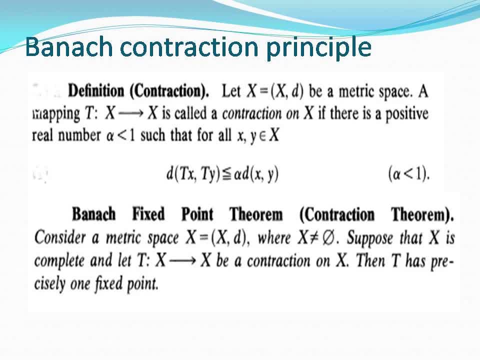 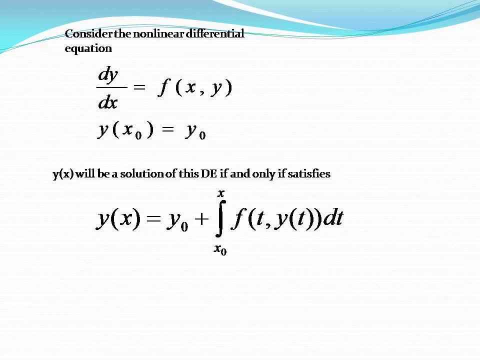 principle which says that t has exactly one fixed point. Now where this fixed point is applied. So we can consider a nonlinear differential equation. So in applications we can have differential equations. which represents the real life problem. So in applications we have differential equations of any order. 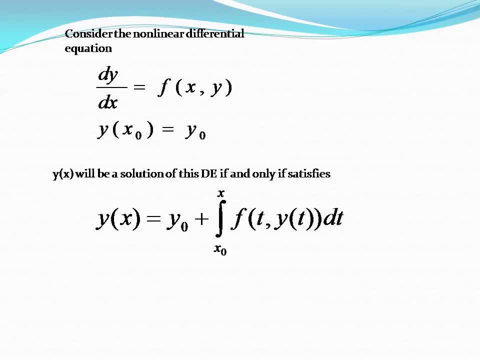 But here we are going to consider a nonlinear differential equation of first order, and that is dy by dx equal to f, y, with y of x0 equal to y0 as the initial condition condition, Because in various applications the problem will be formulated as a differential. 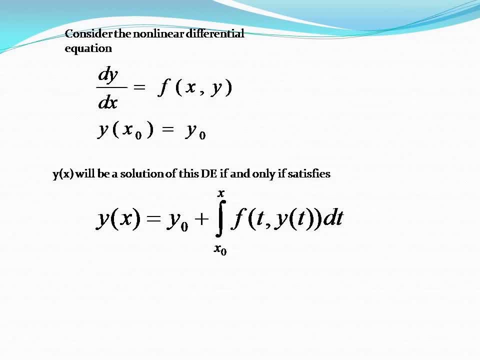 equation and we have to solve the differential equation and the solution will be a continuous function. So y of x will be a solution of this differential equation if and only if, it satisfies y of x equal to y naught plus x naught, t x, f of t comma, y of t dt. So if 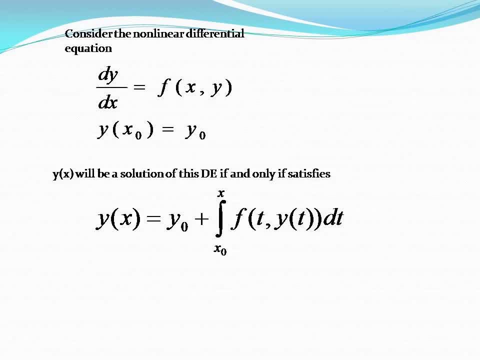 it satisfies this. this is called integral equation. then we say that y is also a solution of the above differential equation. So now we are going to use contraction principle to say that this differential equation is a solution. So we define a map t of y, of 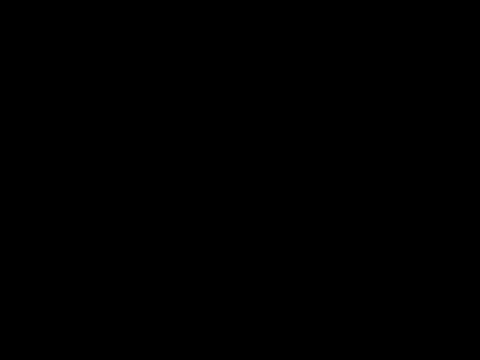 x equal to y naught plus x naught, t, x, f of t, comma, y of t, dt, Then we can observe that the fixed set point of this map, that is, if t of t, y of x equal to y of x, then that fixed set point will be a solution of the differential equation. 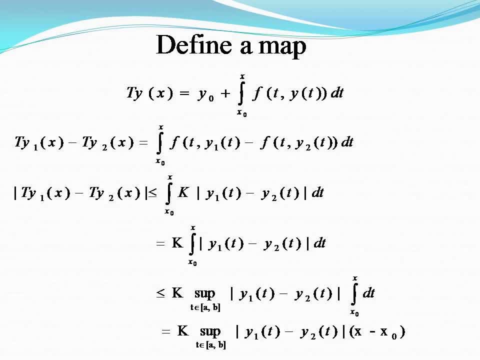 Now we are trying to find the distance between two functions. So here y of x is a function. So if y 1 is a function and y 2 is a function, they are all continuous functions. Therefore the image is also a continuous function and we are trying to find a distance between two. 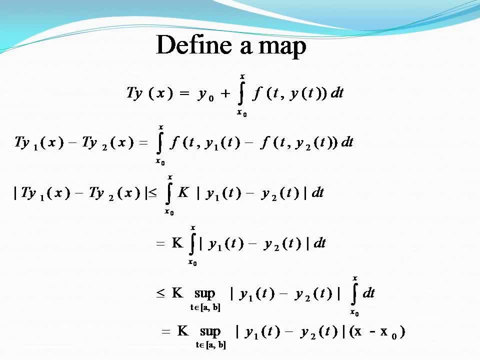 continuous functions, And we know that distance between two continuous functions can be found by determining the supremum of the distance between the function at all the points. So we have modulus of t, y, 1 of x minus t of 2 of y, onlyним Volts. 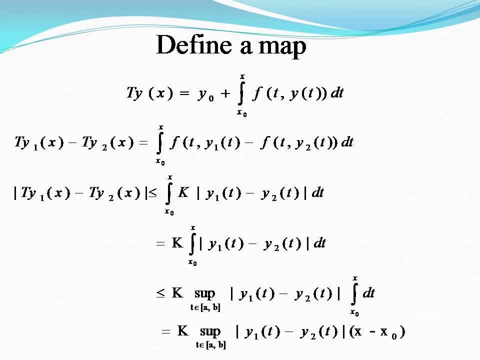 v of x less than equal to x, naught t of x- k into modulus ofy 1 minus y, 2 of t. Here k is the Lipschitz constant. So this is the condition that that f should satisfy. That is f of x- y1 minus f of x- y2 less than equal to k into y1 minus y2.. 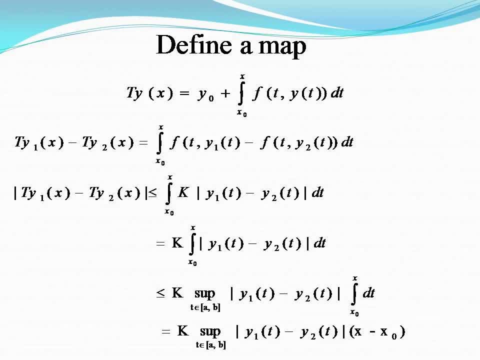 So only if the f satisfies the Lipschitz condition we can have a contraction here. So modulus of ty1 minus ty2 of x less than equal to k into x0 to x. modulus of y1 of t minus y2 of t- dt. 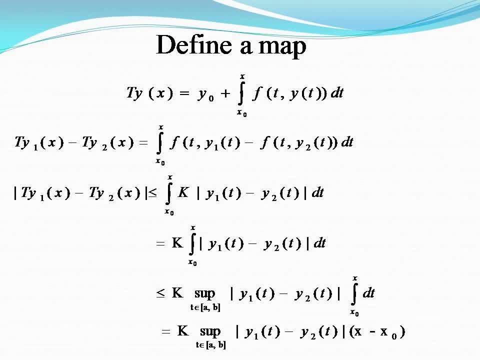 And we can take the supremum on the right hand side. Therefore we can take the supremum outside the integral. So finally we get modulus of ty1 of x minus y2 of x is less than or equal to k into supremum of y1 of t minus y2 of t, into x minus x0.. 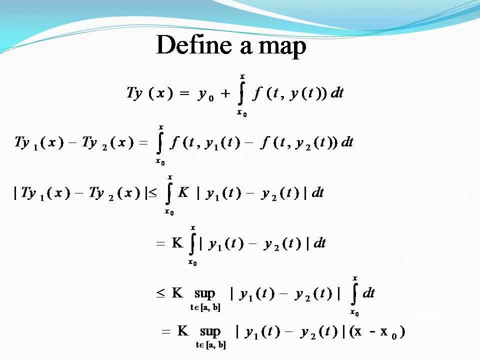 So the distance between these two maps, that is ty1 and ty2, is less than or equal to k into modulus of y1.. y1 of t into y2 of t. So distance between ty1 and ty2 is less than or equal to k into distance of y1 comma y2.. 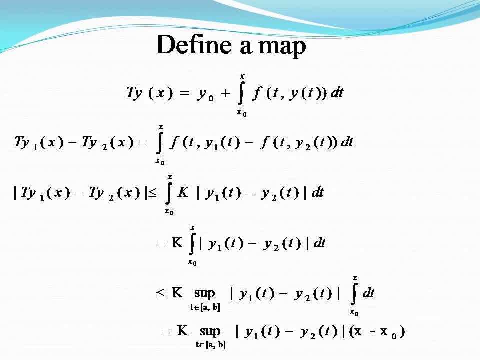 Therefore, by Banach contraction principle, this function, ty of y of x, defined as such as a fixed set point, And that fixed set point will be a solution of the differential equation. The, depending upon k, the fixed set point can may exist only for a particular interval. 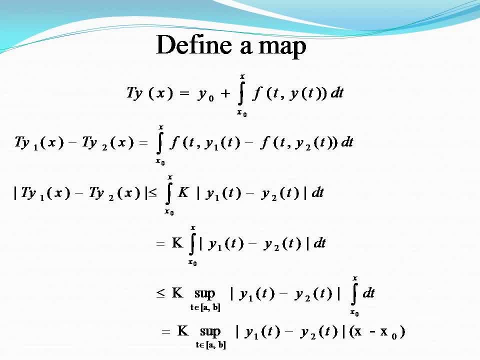 And depending upon f of x comma y, that interval also can be enlarged so as to get a solution for a large number of interval. So this is how we apply the Banach contraction theorem to find a solution for a first order differential equation. 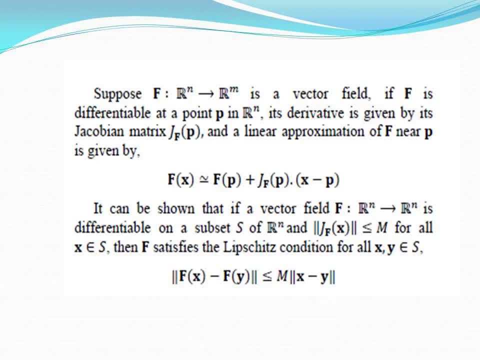 Fixed set point technique Can also be used in determining a unknown function which represents some signal or some phenomenon. Consider a function: f from r power n to r power. m is a vector field. If f is differentiable at a point p in r power n, then its derivative is given by its Jacobian matrix j f of p at a point p. 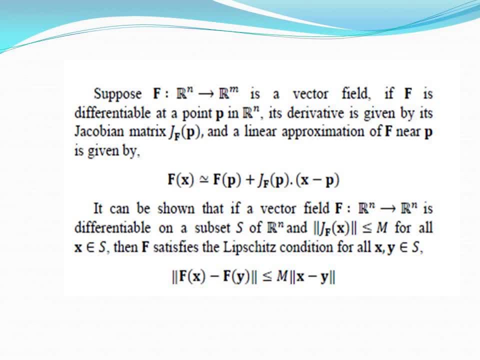 And it is a linear approximation of f near p is given by f of x. So f of x is approximately equal to f of p plus j f of p into x minus p, That is, f of x minus f of p is approximately equal to j f of p into x minus p. 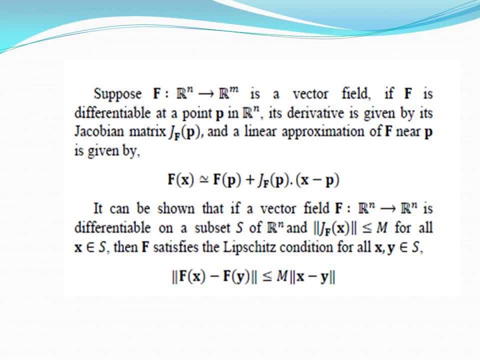 It can be shown that if a vector field, f, from r power n to r power n, is differentiable on a subset s of r power n, And if modulus of j f of here j f, x is a Jacobian matrix, Because f is a function from r, 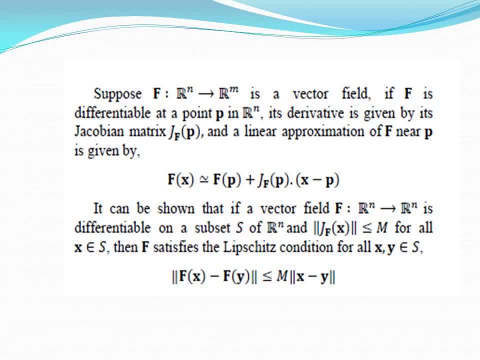 It is a function of n, It is a function of n variables And its image contains m components. Therefore, the Jacobian matrix will contain m cross n entries. We are taking into all the combinations of partial derivatives into account and forming a matrix. 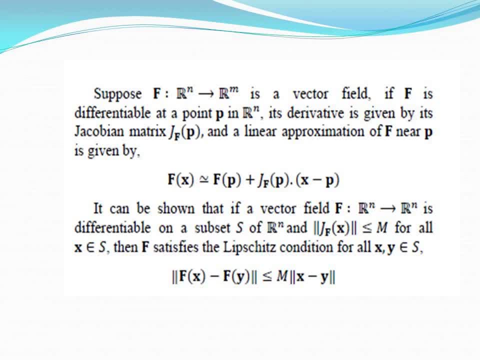 That is called a Jacobian matrix. And if the norm of the Jacobian matrix less than equal to m, for all x belong to x, Then f satisfy the Lipschitz condition, for all x comma y belong to s. That is norm of f of x minus f of. 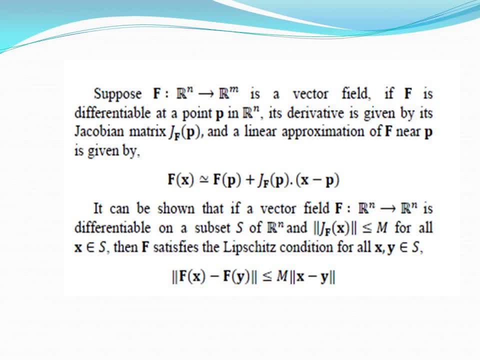 y less than equal to m into norm of x minus y. So again we require as the differential equation that f should satisfy the Lipschitz condition. So once when f satisfies the Lipschitz condition, we can apply this to find whether this function f has a fixed point or not. 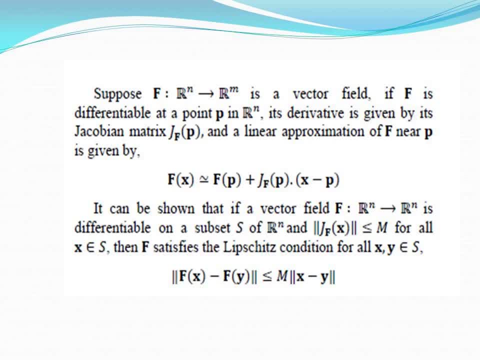 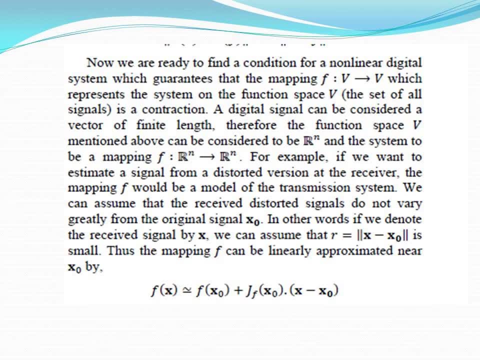 Because now we are ready to find a condition for a non-linear digital system Which guarantees the mapping f from v to v, which represents the system on the function space v. So here v is the set of all signals, So each signal can also be represented by a continuous function. 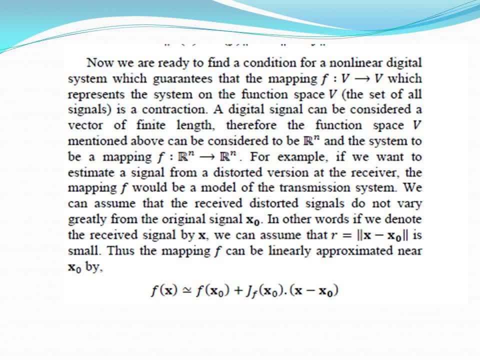 It can also be in the waveform: A digital signals can be considered a vector of finite length. So here we are interpreting a digital signals and giving a mathematical meaning to it. So a digital signal is considered as a vector of finite length. Therefore the function space v can be considered to be r power n and the system to be a mapping from r power n to r power n. 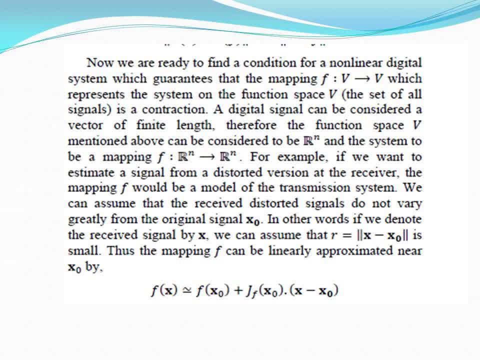 So if you want to estimate a signal from a distorted version of the receiver, So at the receiver we are getting a distorted version of the original signal. So here we are not getting a original signal but a distorted version of the original signal, But it is approximately closer to the original one. 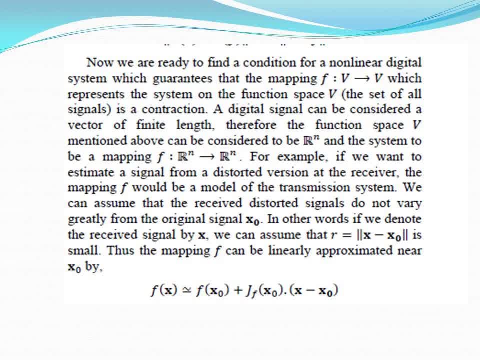 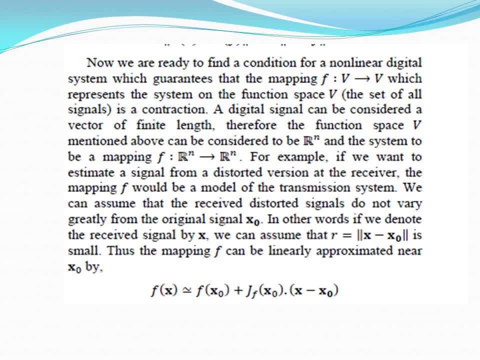 Hence the Jacobian matrix of f at the point x0,. of course, here the Jacobian matrix becomes a n cross n matrix. So the derivative of f is j of x can be considered to be constant in the subset of r power n, where our signals lie. 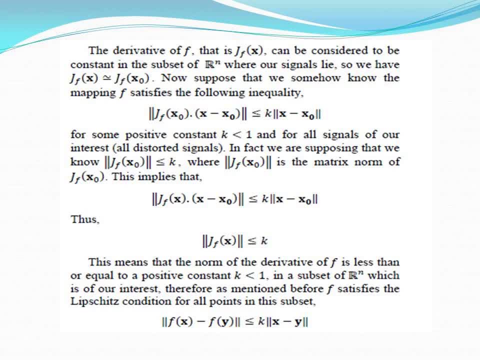 So we have: j f of x is also equal to j f of x0, because x is closer to x0 and j f is linear. Therefore, we can assume that j f of x is approximately equal to j f of x0.. Therefore, we can assume that j f of x is approximately equal to j f of x0, because x is closer to x0 and j f is linear. 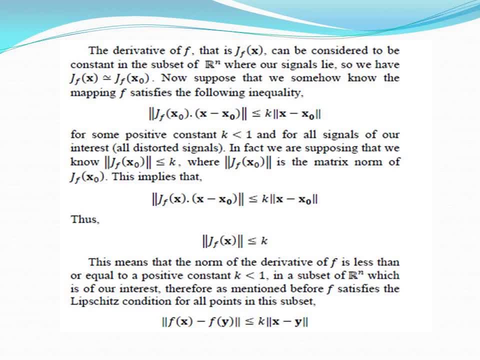 of x0.. Now suppose we know that f satisfies the inequality norm of jf of x0. dot x minus x0, less than equal to k, into norm of x minus x0.. Here by norm we mean the distance between any two points in r power n. So the distance between any two points in r power n is given. 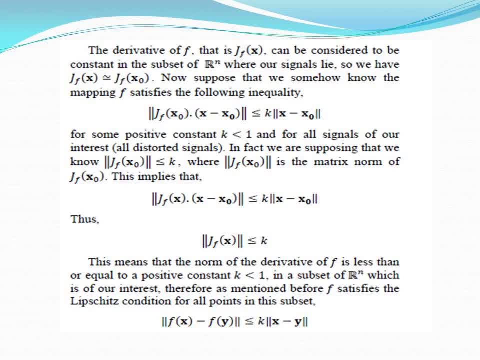 by the usual Euclidean distance, So if f satisfies this condition, and for all signals of our interest. so whatever distorted signals we get in fact. so what we are expecting is that we know that norm of jf of x0 is less than equal to k, where norm of jf of x0 is: 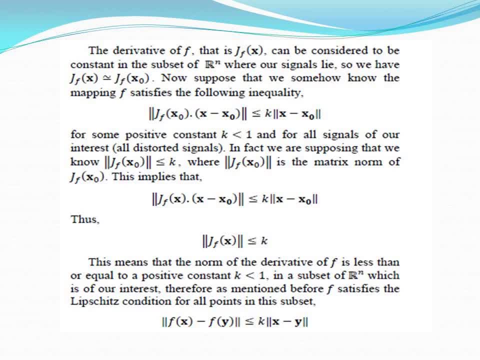 the matrix norm of jf of x0.. So, which gives a relation, that norm of jf of x, norm of jf of x, norm of jf of x0 is less than equal to k. So we know that norm of jf of x0 is: 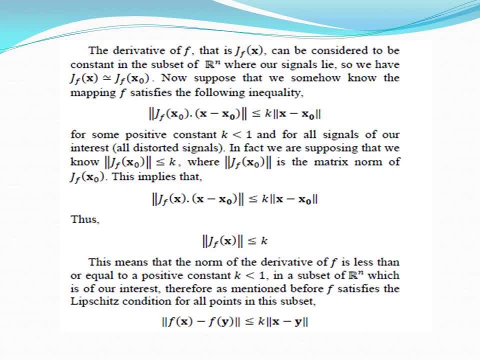 less than equal to k into x minus x0. less than equal to k into norm of x minus x. Therefore we have the desired condition: norm of jf less than equal to k. That means that norm of the derivative of f is less than or equal to a positive constant k less than n. So 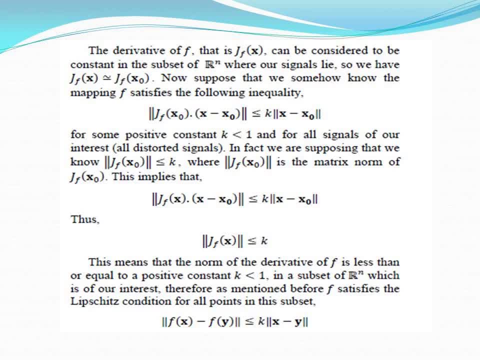 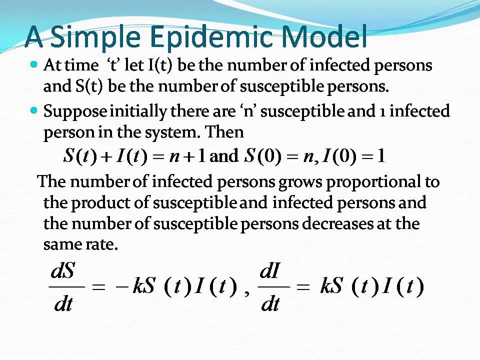 this gives. this makes f as a contraction, So as f is a contraction, by Banach contraction theorem we are able to get that f has a fixed point, and the point at which f has a fixed point will be our original signal, because it does not have any distortion. Now we move to other applications, which uses: 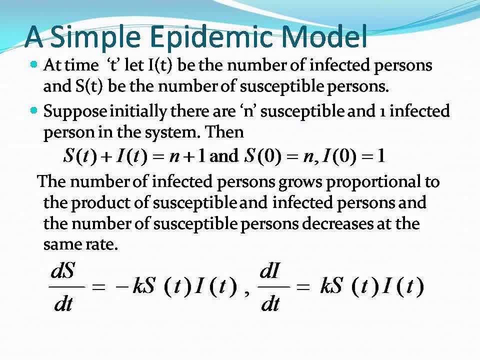 differential equations and integral equations. Here we consider a simple epidemic model, an epidemic model where the disease spreads among a population. here the size of the population is n plus 1.. So at any time, t, let I of t be the number. 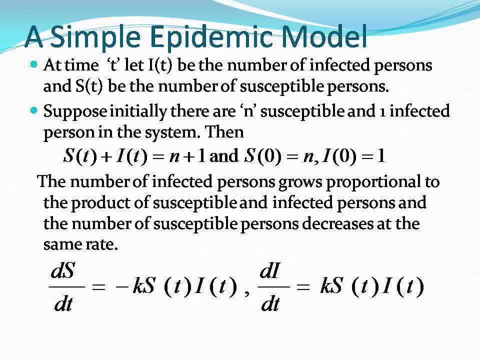 of infected persons and S of t be the number of susceptible persons. So I of t denotes the number of infected persons who are already infected by the disease, and S of t is the number of susceptible persons, So the susceptible persons means those who are likely to get infected. 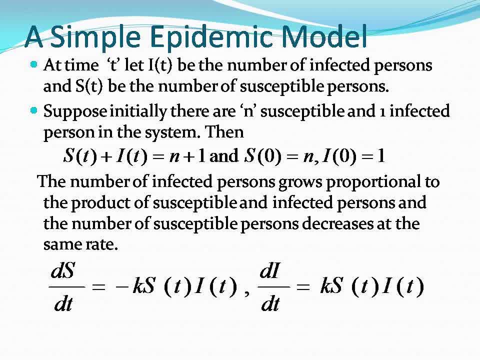 by the disease. This likelihood may be because they are near to the infected persons or because inevitably the disease will spread to all the populations in the system. So the size of the population is n plus 1 and suppose initially there are n susceptible and 1 infected. 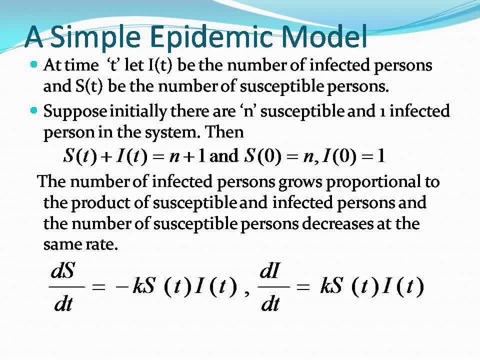 person in the system. then we have the simple equations: S of t plus I of t equal to n plus 1.. Because the total size of the population is n plus 1 at any given point of time, s of t plus i of t equal to n plus. 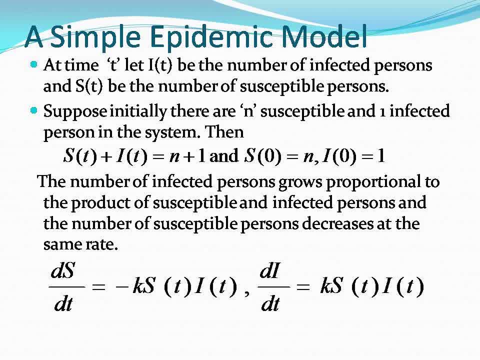 1 and initially the starting, we have only one infected person. so s of 0 equal to n and i of 0 equal to 1. now the number of infected persons goes proportional to the product of susceptible and infected persons. so depending upon the number of susceptible persons and infected persons, the 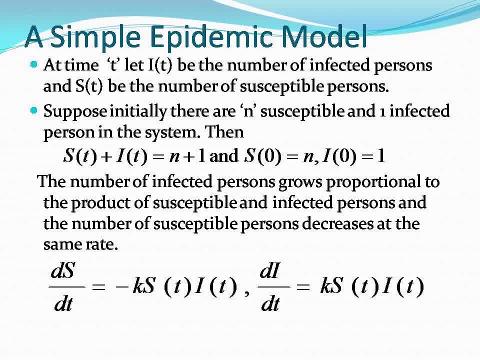 number of infected persons grows up because normally a time increases, the number of infected persons will grow till a particular time, so depending upon the already available infected persons. if there are few infected persons, the number of the growth will be slow. if there are more infected persons, the growth 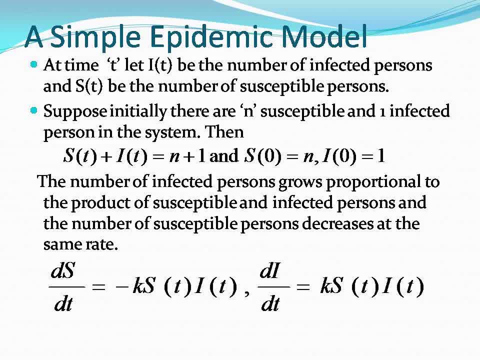 will be slow and if there are more infected persons, the growth will be slow and if there are, will be large. So the number of infected persons grows proportional to the product of susceptible infected persons, and the number of susceptible persons decreases at the same rate. It is also proportional to the product of susceptible infected persons, but here 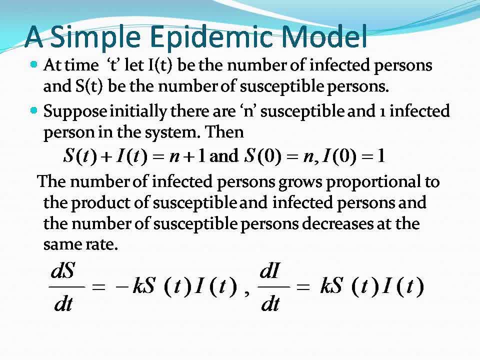 it decreases. So we have to attach a negative sign. So we have the equations ds by dt equal to minus k into s of t, i of t, and di by dt equal to k into s of t, into i of t. So if 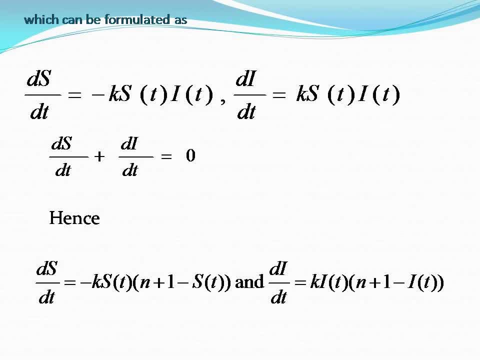 we add these two equations. if we add ds by dt and di by dt, both the terms of right-hand side cancels out. So we have ds by dt plus di by dt equal to zero. and but already we know that s of t plus i of t equal to n plus 1. 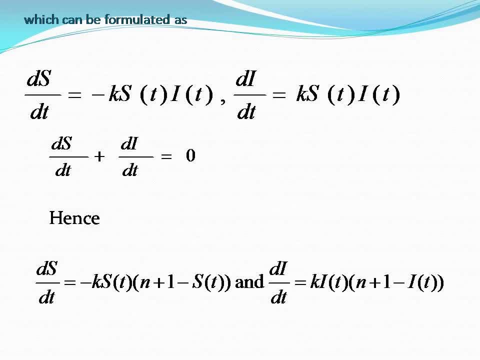 so we can replace i of t by n plus 1 minus s of t, and here we can replace s of t by n plus 1 minus i of t. so why we are replacing is because now we have s is the only variable, so ds by dt equal to minus k into s of. 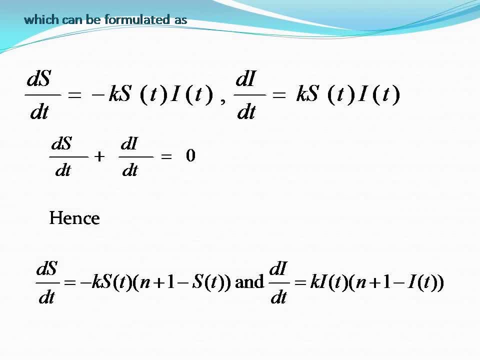 t n plus 1 minus s of t. now this is the first order non-linear differential equation because it is proportional to the right answer. we have the order of s of t square, so it is the first order non-linear differential equation. similarly, di by dt equal to k into i of t n plus 1 minus i. 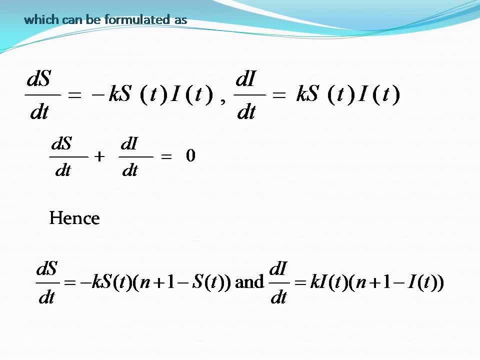 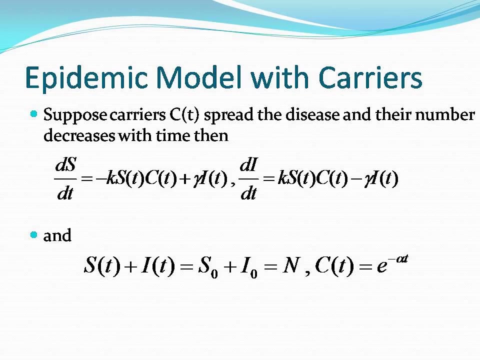 of t is also a non-linear, first order differential equation. so we can understand how the first order, non-linear differential equation is formulated in a epidemic model. now if we in in this model, if we also have carriers, so carriers means those who are capable of carrying the disease, so they can be also silent carriers. so suppose carrier c of t spread the. 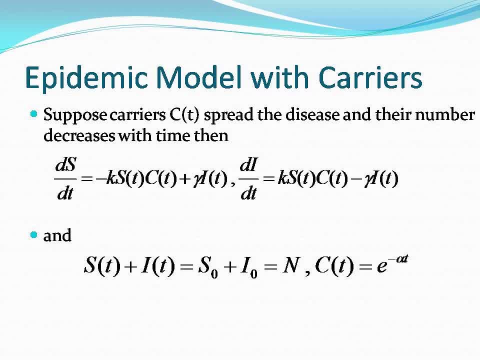 disease and the number decreases with time, because these carriers can be easily identified and eliminated, so they may not be infected, but they will act as carriers to just spreading the disease. so then we have to add a corresponding term, because the growth of the susceptible persons is proportional to the the population of the infected persons. so depending on the population, 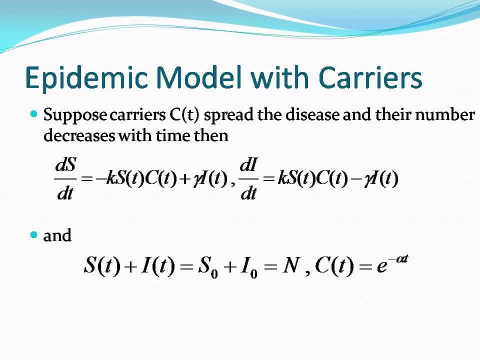 of the infected persons, we have the growth of the susceptible person. so here we add a factor gamma into i of t and similarly the growth of the infected persons is negatively proportional to the growth of the the population of the infected persons, because in this case we are identifying the carriers and there we are eliminating them. therefore, depending upon the 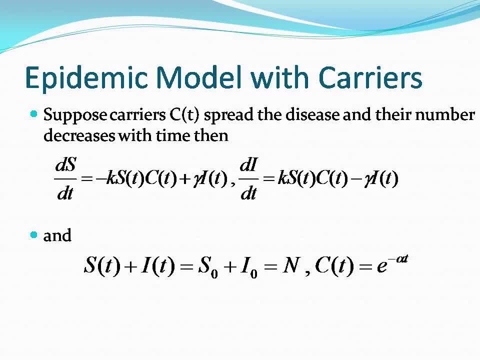 population of the infected persons. we have the. the ds by dt is proportional to the population of the infected persons, but here it is. but it is proportional to the product of susceptible persons and carriers. so here, instead of the product of s of t and i of t, we get s of t into c of t. so ds by dt. 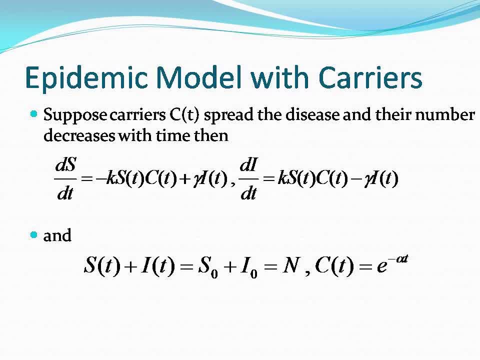 equal to minus k into s of t, into c of t, plus gamma into i of t. and similarly, di by dt equal to k into s of t, into c of t, minus gamma into i of t. so this is the growth itself and that we can use it to define it as direct Human Emigmat. Residential Casual. 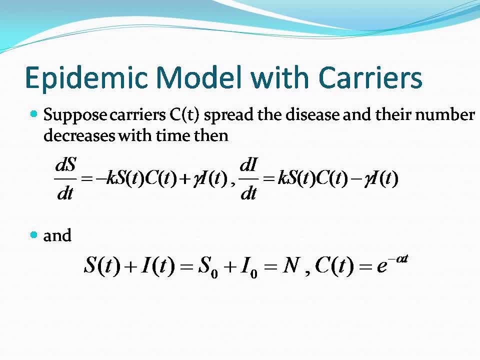 of t. This c of t also can be determined because the growth of the rate of growth of this carriers they are negatively proportional to the population of the carriers itself. So the c of t is given by e power minus alpha t, where, as t tends to infinity, the c of 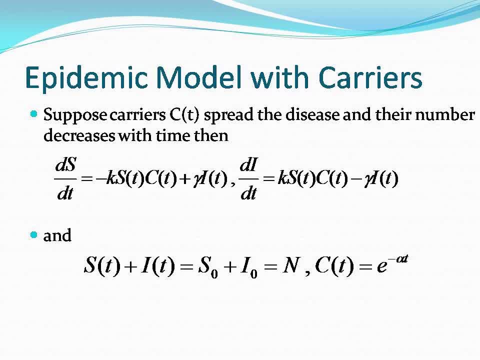 t goes to zero, And also s of t plus i of t equal to s naught plus i naught, equal to capital N. Here the size of this population is capital N. So here you can modify this epidemic model when there are carriers and therefore we can form the differential equations. 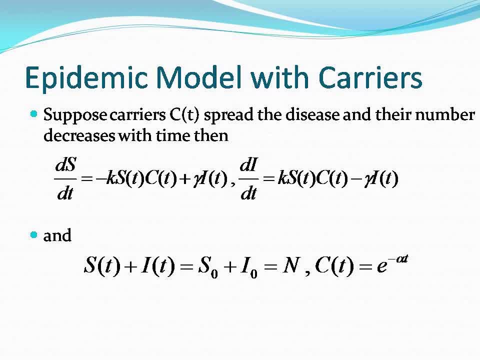 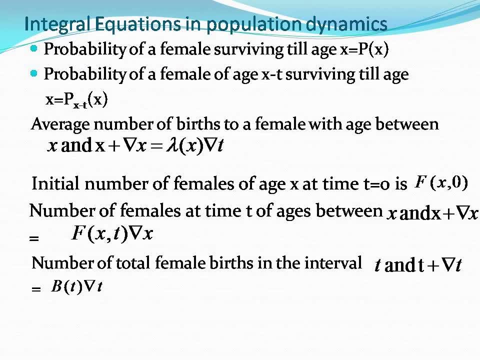 of first order. non-linear differential equations, Integral equations in population dynamics. In population dynamics we study why population structure changes with respect to birth rate, death rate, according to the age of the population. So here we have various probability factors which helps to study the population dynamics: Probability of a female surviving till age x. So here 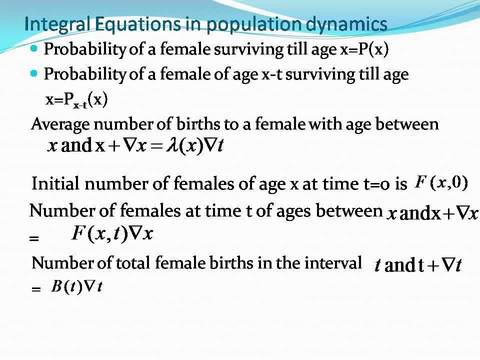 we want to analyze the female birds. So probability of a female surviving till age x is given by p of x and probability of a female of age x minus t surviving till age x. So what is the probability of a female of age x minus t surviving till age x? So she has to live. 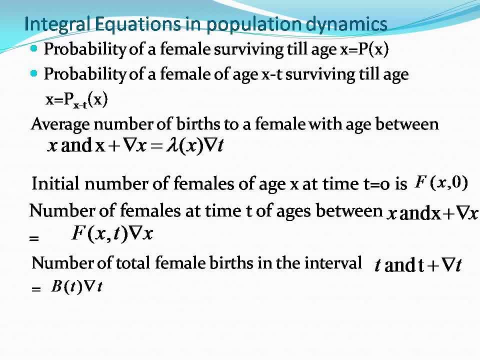 t years to survive till age x. So what is the probability? It is given by p of x And average number of birds to a female with age between t and age x is given by p of x. So the probability of a female of age x between x and x, plus delta x, is given by lambda x. 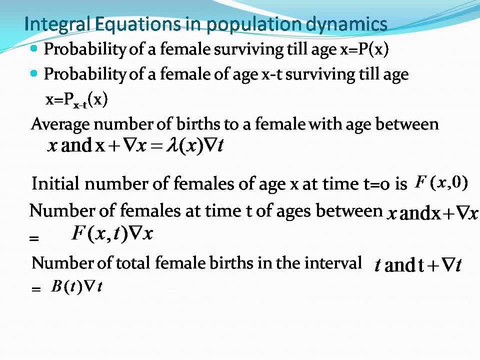 into delta t. So this is the how many female birds can happen through a female. So when a female gives birth to a female, so how many female birds can happen through the present female who are of reproductive age group. So this is the average number of birds to 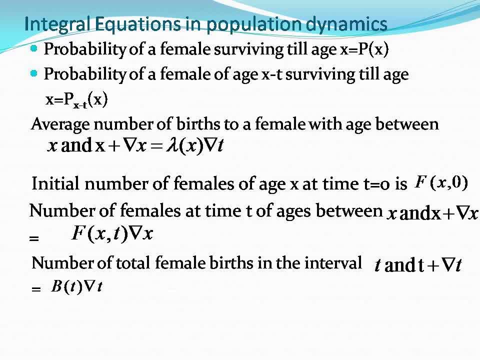 a female with age between x and x plus delta x is given by lambda x into p of x. So the delta t And initial number of females of age x at time t equal to 0, is given by f of x comma 0.. In general, f of x comma t is a function which gives the number of females. 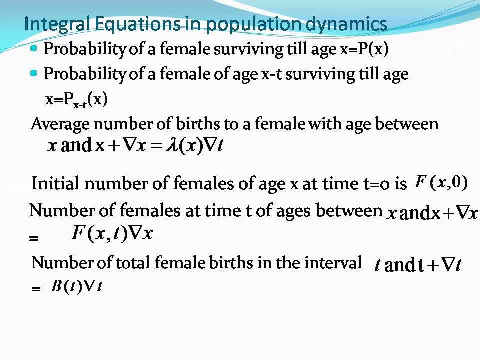 of age x and time t. So as a initial condition we have the initial number of females of age x at time t, equal to 0, is given by f of x comma 0. And similarly, number of females at time t of ages between x and x plus delta x is given. 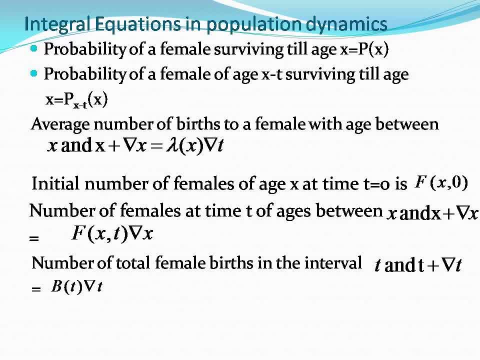 by f of x, comma t into delta x. And finally, total number female birds at time t is given by b of t. So b of t denotes total number of female birds in 10 to 12 minutes time t. And so, if you analyze the time interval, so everything we are able to analyze only. 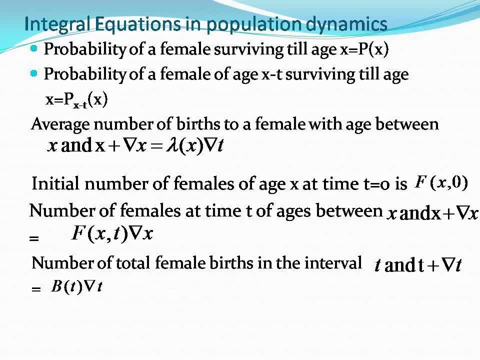 in the time interval, So between time t and t plus delta t, the total number of female birds is given by b of t into delta t. So here we have two cases: the relation between f, of and the other variables. If x is less than or equal to t, suppose 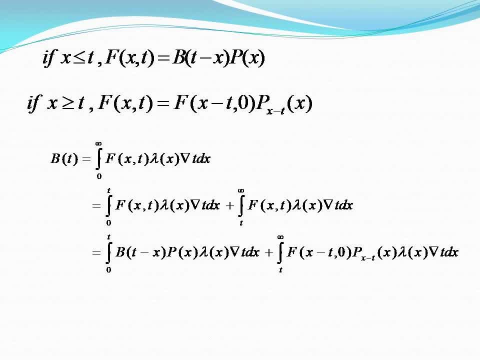 x is less than or equal to t, then f can be written as b of t minus x into b, Because we know that f is nothing but total number of females of age, x at time t. So this is equivalent to calculating the. total number of females. what is of that age? t was b. Let us connect the rules. that is, in this particular case, if p equals to alpha, rep mean alphaeta in the operator million. that remains the produce of the NGC, because p equals to minus beta, plus delta, t and alpha. 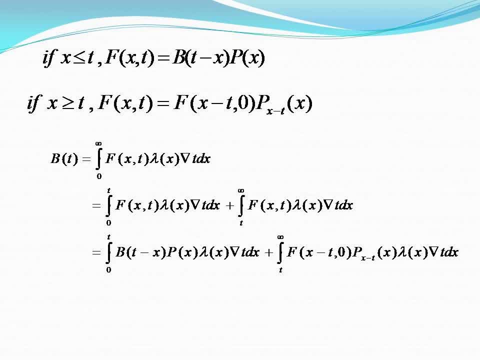 equals x. ifulse is really bring a solution to the total number of females. so what happens thencroses, and don't always think that we are able to had well shown theition of échanges. total number of female births at time: t minus x and those who have survived for x years. 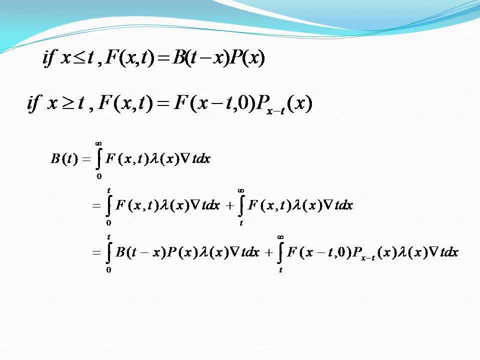 So any female birth at time t minus x and surviving x years can be taken into account of T minus x times female of age X at time t. So f of x comma, t equal to B of t minus x into multiplied by p of x. 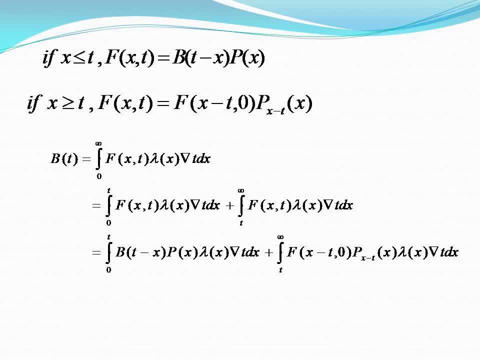 So why we are multiplying by p of x? Because among the female births that has happened at time t minus x. we do not know how many of them have survived till x years. So that is given by the probability term p of x, or that is why multiplying this probability 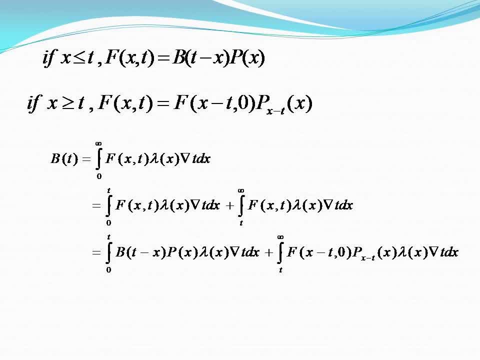 term p of x, So f of x. comma t equal to T minus x. Ok, equal to b of t minus x into p of x. So this is valid only for x less than or equal to t. If x is greater than or equal to t, f of x. t is equal to f of x minus t, 0 multiplied. 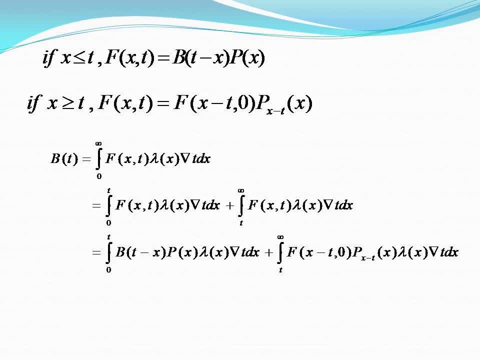 by p of x minus t of x, Because f of x, t is the total number of females of age x at time t. it is equivalent to calculating the total number of females of age x minus t at time t equal to 0. And they have to survive for t years. So that is given by the probability. 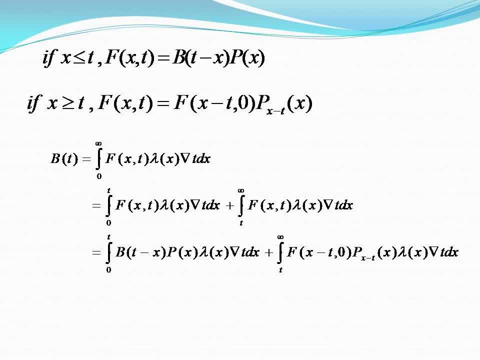 of a female of age x minus t and surviving till age x, So surviving for t years. When you multiply this probability, we get f of x t equal to f of x minus t, comma 0, multiplied by p of x minus t of x, Now b of t. So b of t is the total number of female birds. 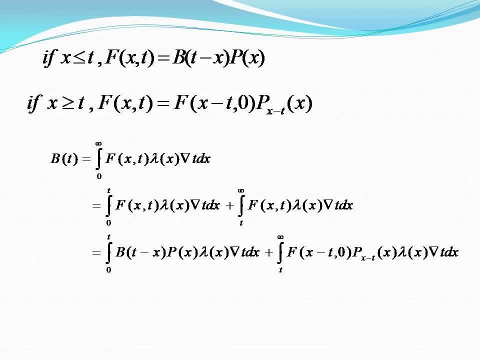 at time t. So at a particular time, if you want to fix the time t, you fix time t At that particular time. if you want to find how many female birds have happened- so that is equivalent to first- we have to find out f of x comma t. So f of x minus t is equal. 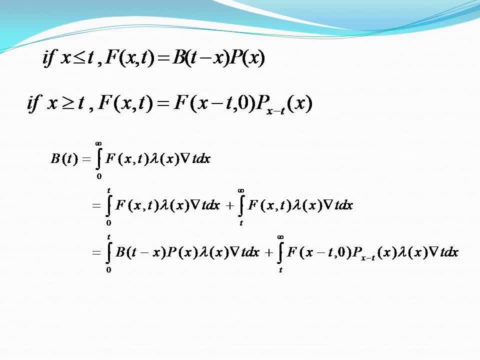 to 0. That is total number of female of age x at time t, Because t is fixed. So at time t how many female are present at age x? It is given by f of x comma t And we are multiplying. 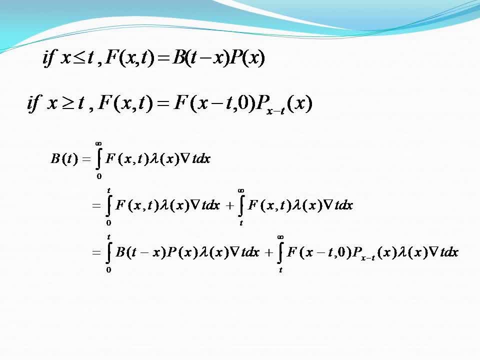 by lambda x, Because among those females of age x at time t, only some of the females, Only some of the females give birth to a female birth. So that is given by lambda x. So that is why lambda x is nothing but average number of births to a female with age between x and x, plus delta x. 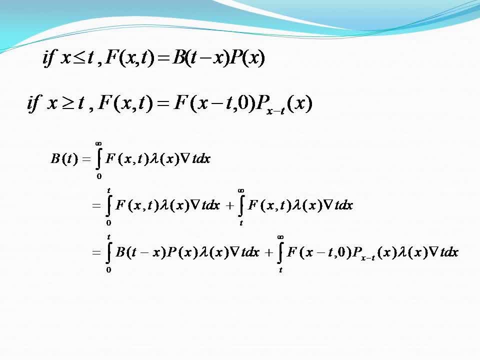 So that is given by lambda x into delta t. So when we multiply by lambda x into delta t, we get among those females who are currently present among them, how many of them will be giving birth to a female? So that is given by lambda x into delta t. So b of t is integral 0 to infinity, because b of t is the total number of female births at time t. So we have to take all the ages into account. 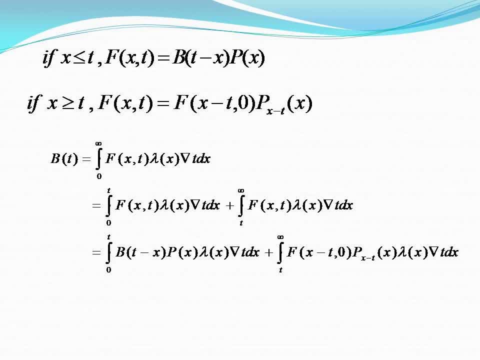 So actually, here x will have an age group of reproductive age group, So lambda x. if x is outside the reproductive age group, lambda x can be taken to 0. So here though we are integrating from 0 to infinity. actually, the integral is from some finite interval, where outside the finite interval is nothing but the reproductive age group. 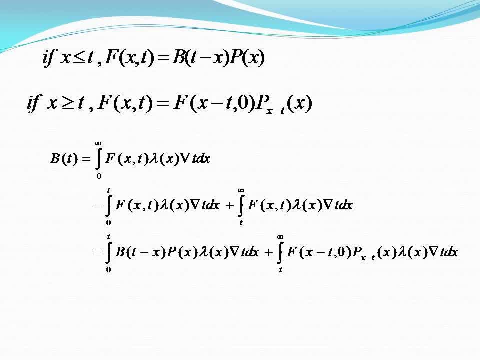 As I demonstrate the experiment, the female of those reproductive age groups will be giving birth to a female. So this integral can be split into two integrals: Integral 0 to t, f of x, t lambda of x, lambda t, dx, plus integral t to infinity with the same integrand. 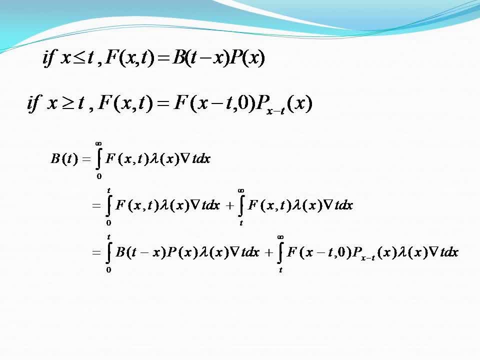 And now applying the above two equations for x less than equal to t and x greater than equal to t. That is why we have split the integral into two integrals. So now applying the above integrals for x greater than equal to t by adding in on one plus two integrals. So, for example, here we have three integrals. 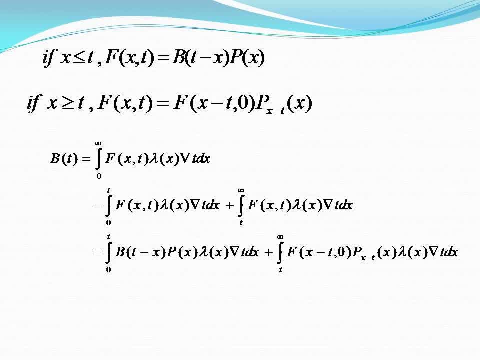 x less than or equal to t and x greater than or equal to t. we replace f of x- t by b of t minus x into p of x, where x less than or equal to t, and we replace f of x- t equal. 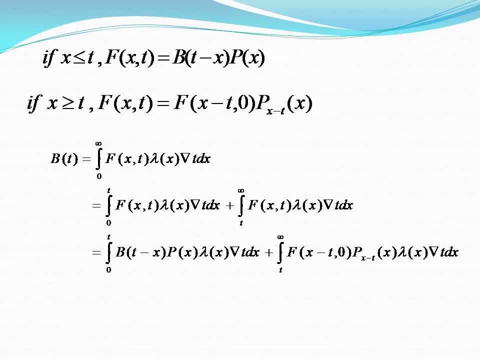 to f of x minus t, comma zero into p of x minus t of x for x greater than or equal to t. So finally we get b of t equal to integral zero to t. b of t minus x. p of x lambda is: 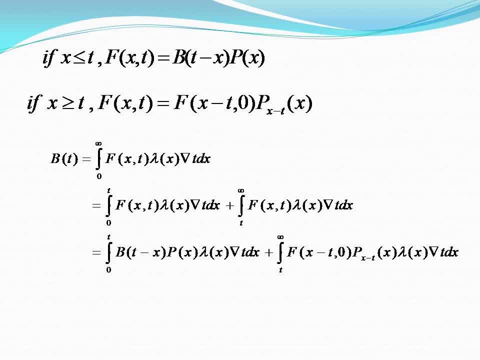 delta t dx plus integral t to infinity, f of x minus t, comma zero, p of x minus t of x, lambda x, delta t dx. So here you can see that this equation is an integral equation. So, these integral equations, what are the knowns, These probabilities, p of x and p of? 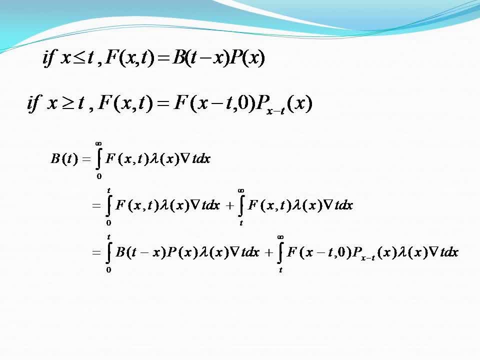 x minus t of x can be found from the statistical analysis of the census data. And also this: f of x minus t, comma zero is nothing but the total number of females of age x. So here x minus t is a variable. You can replace this variable by another variable. 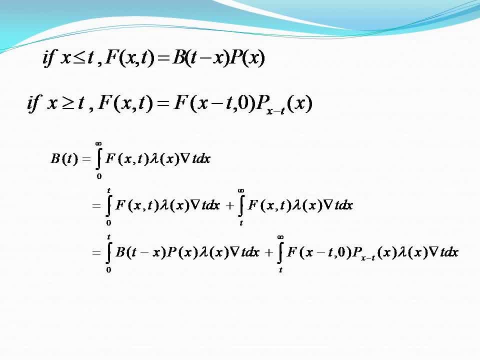 So it is nothing but f of x comma zero or f of y comma zero, where we have to find the total number of females at time t equal to zero. This also can be got from the census data or any population data. So here all the other terms are knowns. 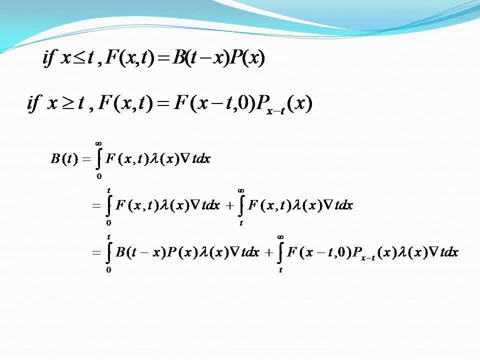 Except b of t minus x And the left hand side also, we have b of t. So this is an integral equation And when we solve this integral equation we are able to determine b of t. So this is how integral equation plays a role in population dynamics. 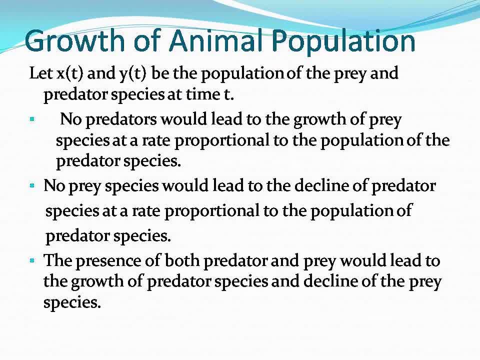 Now we analyze the growth of animal population from the population of prey and predator species. We know that The growth of prey and predator species is quite crucial to the ecological balance, So both prey and predator species should be present at the same size or prescribed size. 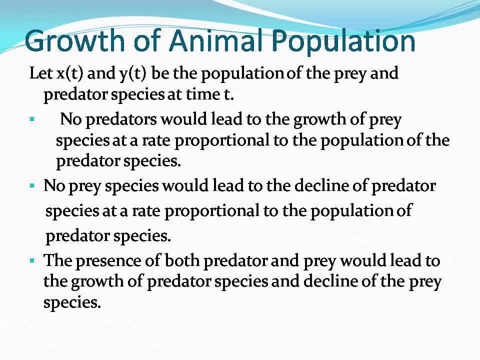 Then only there will be an ecological balance. So here we consider x of t and y of t as a population of prey and predator species at any given time, t. So X of t Is the population of species, and why you are free- the population of predator species at any given time, t. 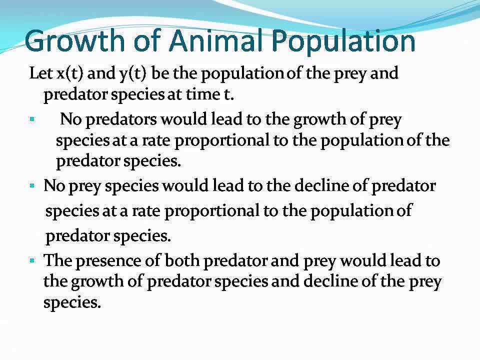 Suppose there are no predators, then this would lead to the growth of prey species at the rate proportional to the population of the predator species. So suppose we have no predators, then the prey species will grow rapidly because, as there are no predators, will guarantee its survival and it will grow rapidly. and this 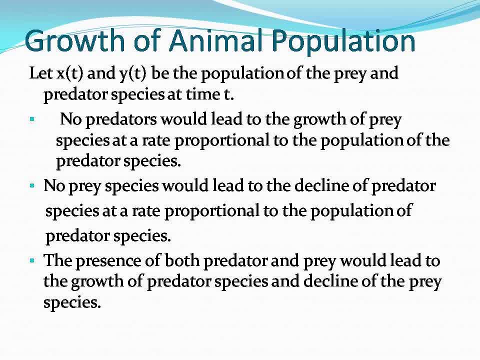 rate will be proportional to the prey species. So the rate of growth of prey species will be proportional to the population of the prey species. Suppose there are no prey species, then this will lead to the decline of the predator species, because the predator depends on the prey for its survival. 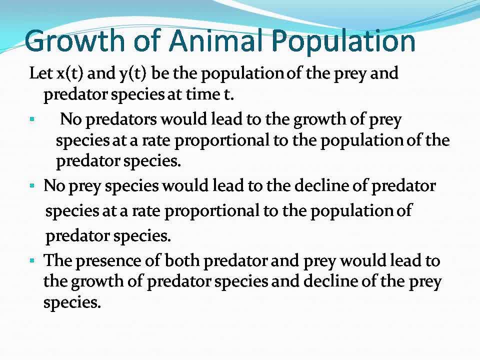 So, and for its food. Therefore, if there are no prey species, then the predators will be starved and this will naturally lead to the decline of the predator species at the rate proportional to the population of predator species. So here the proportion is negative. proportional because according to the present population. 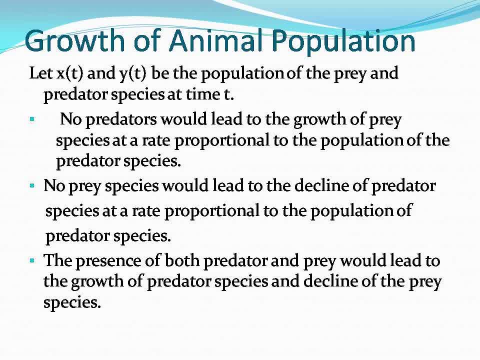 of predator species, the population will decline. and here we have to add a negative sign: The presence of both prey and predator species will lead to the growth of predator species and decline of prey species, Because if both are present, then the presence of both predator and prey species will be. 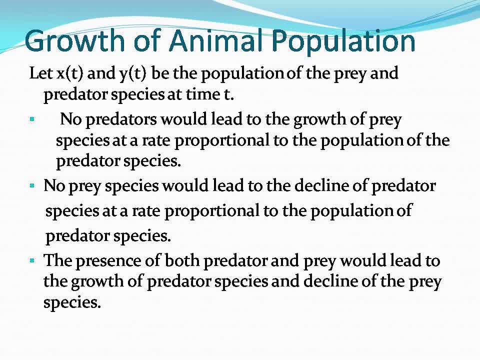 beneficial to the predator species, but it will not be beneficial to the prey species. it will be to the decline of the prey species Because since, as long as the predator is present, the prey species is always in a danger. So how to model this into a mathematical equation? 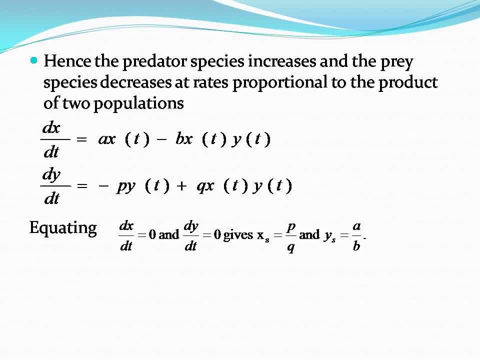 So since the predator species increases and the prey species decreases at the rate proportional to the product of two populations, So already we know that dx by dt, equal to a into x of t, Where x of t is the population of prey species. So the growth of the prey species is positively proportional to the growth of the population. 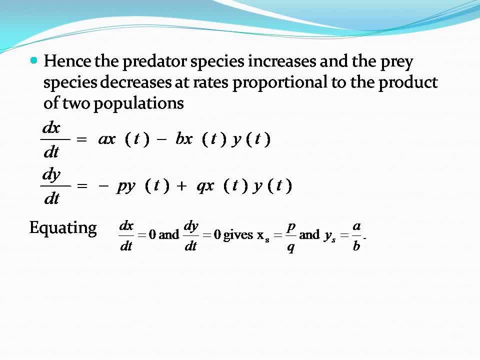 of the prey species. Therefore, dx by dt equal to a into x of t, And here we have an additional term minus b into x of t, into y of t. So this x of t and y of t represents the presence of both prey and predator species. 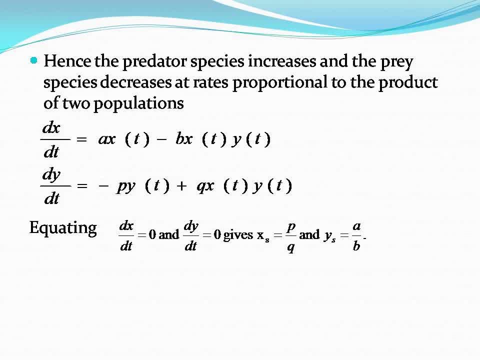 That is why we are multiplying x of t, x of t and y of t. But the growth of prey species is negatively proportional to the product of prey species and predator species. Therefore we are multiplying by a constant b with a negative sign. So dx by dt equal to a into x of t, minus b into x of t, y of t. 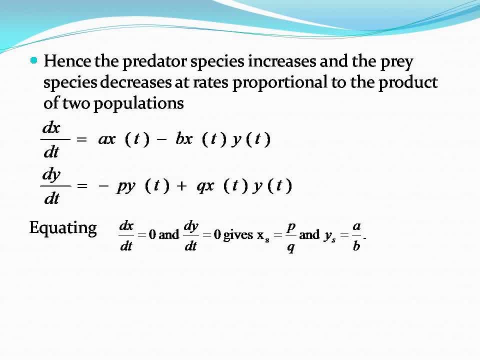 Similarly, The growth of the predator species. The growth of the predator species is negatively proportional to the presence of the predator species, Because simply, if the predator species alone is present, Then it is not beneficial to the growth, Because the more the predator species are present, then there is more demand for the food. 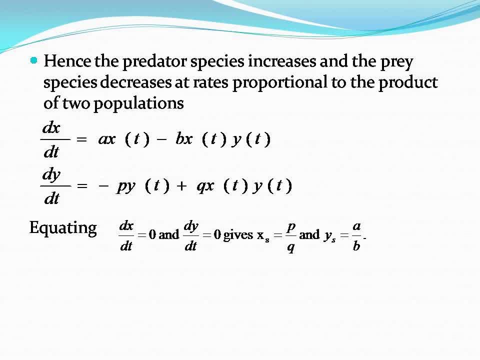 So if there is more demand Then the decline will be further. So depending upon the size of the predator species there will be decline of the predator species. Therefore, dy by dt equal to minus p into y of t. here p is the proportional constant. 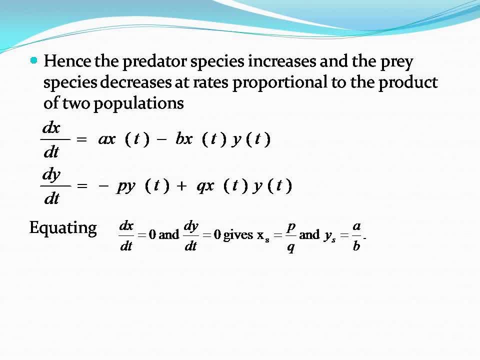 because the growth of the predator species is negatively proportional to the population of the predator species. But when both predator and prey is present, it is positively proportional to the product of the predator species as well as the prey species. Therefore, dy by dt is proportional to x of t into y of t. 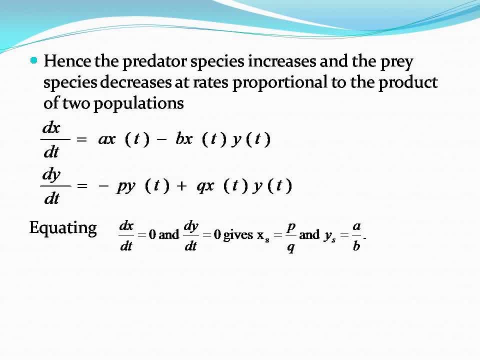 And so we have dy by dt equal to minus p, y of t, plus q into x of t, y of t. So these are the simultaneous equations that govern this population balance between these two species. So now, if you want to find out, 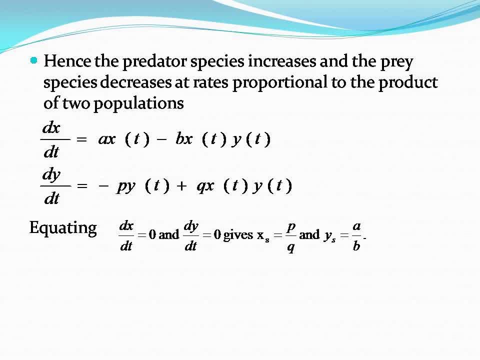 If you want to find the equilibrium size. so what is the correct population size of the prey species and the predator species, where the population of both will not decline and there will not be any rapid growth also? So for that we have to equate dx by dt equal to 0 and dy by dt equal to 0, which gives 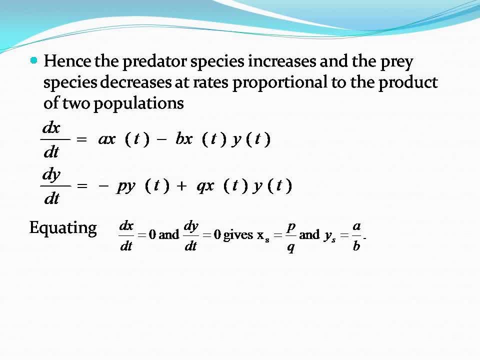 us immediately: xs equal to p by q and ys equal to a by b. So this is the equilibrium size. So this xs equal to p by q and ys equal to a by b are, respectively, the equilibrium size, the equilibrium size of the prey species and predator species. 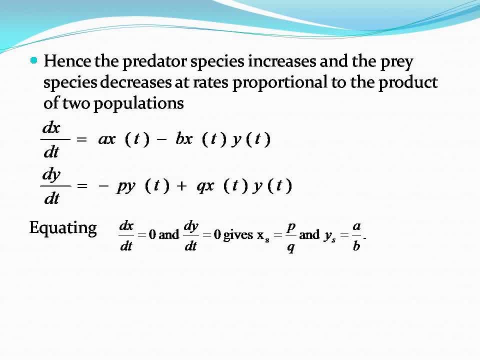 And, of course, this p, q, a and b are proportional constants. These constants we have to determine or we have to derive these constants from the already available population data of these two Species in the past. so what is, what was the growth rate and what was the decline rate? 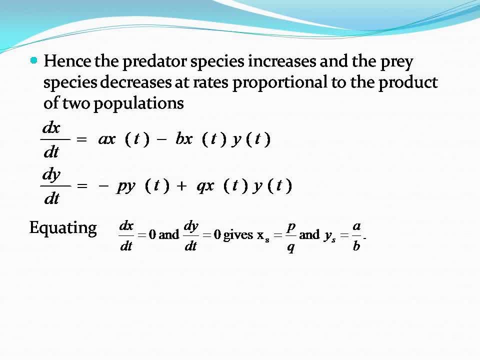 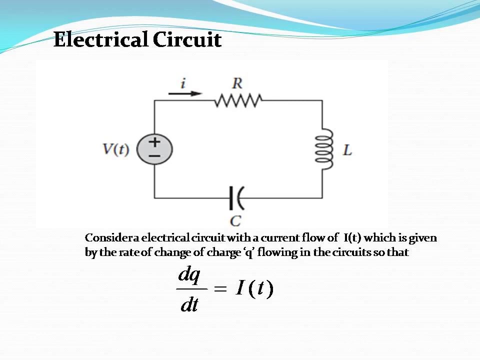 and from these rate we can determine the constants p, q, a and b. So this is the application of simultaneous differential equations to them: Population, growth of prey species and predator species. Now we are going to analyze electrical circuit And see how the flow of current can be analyzed through differential equations. 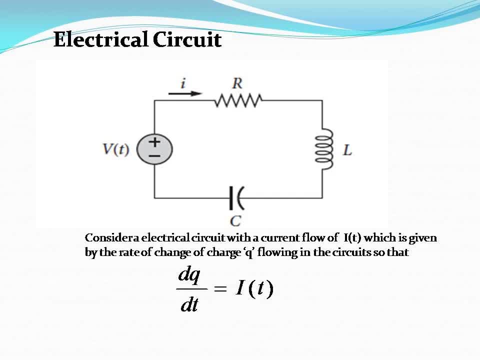 So this electrical circuit contains a resistance r ohms, inductance l and a capacitor c. The current flow I of t with changes with respect to time, is given in terms of amperes. It represents the time rate of change of charge q flowing the circuit. 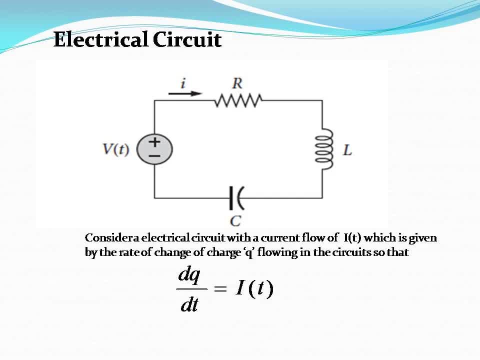 So this is the current flow. I of t, with changes with respect to time, is given in terms of amperes. So since I of t is the rate of change of the charge q, the I of t is given by dq, by dt equal to I of t. 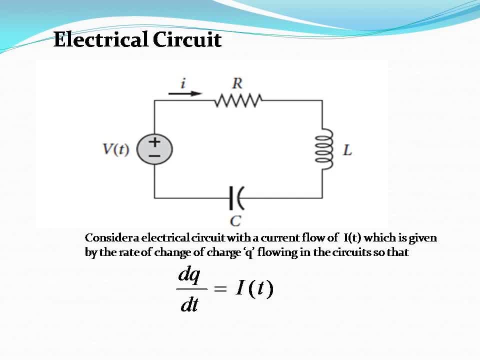 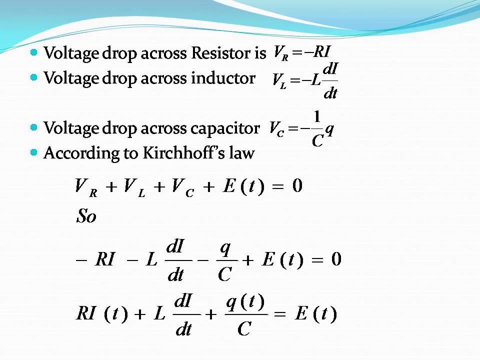 Now, when analyzing the voltage across the circuit, the resistance is given in ohms, r ohms, the resistance of r ohms of the circuit and the voltage drop across the resistance is given by r ohms, Since this is the speed of this circuit. this возer is represented by the şeyler. 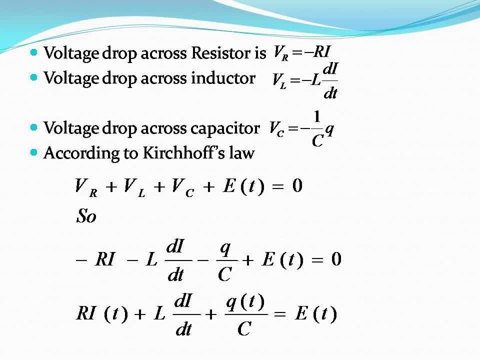 we get asΔ Dr. that will therefore be given by the llegarian모 r into I. Since this is the voltage drop, it is written as minus r into I, And there is also the inductance of the L Henry s, which produces the potential voltage. 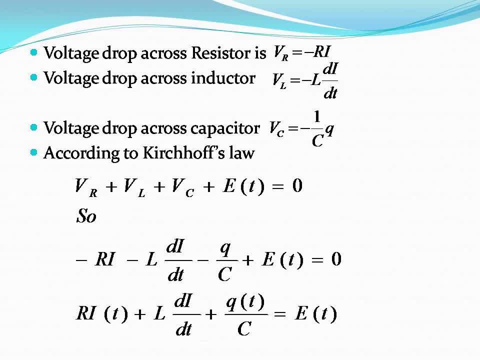 drop of L, Han And the voltage drop across a capacitor is given by minus 1, by c into q. Now for doubt, we will get RI. We can now use thisAr tropic As fifth equation. all these voltage drops are balanced by the battery, which produces E volts. So according 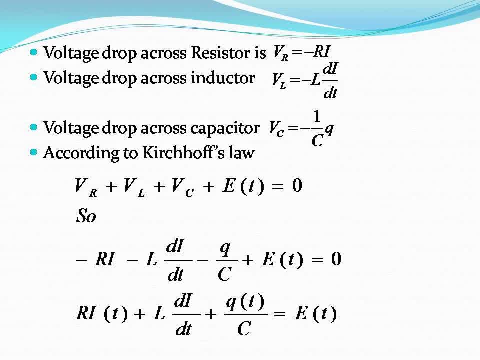 to Kirchhoff's law, the algebraic sum of the voltage drops around the closed circuit is zero. Therefore we have E of t minus R into I of t minus L, into di, by dt plus 1, by c, into q of t equal to zero. So, taking these three terms to the other side, we have R, i plus. 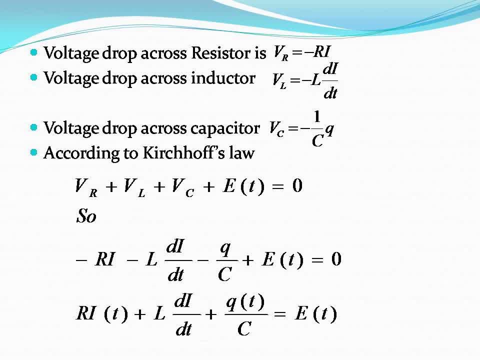 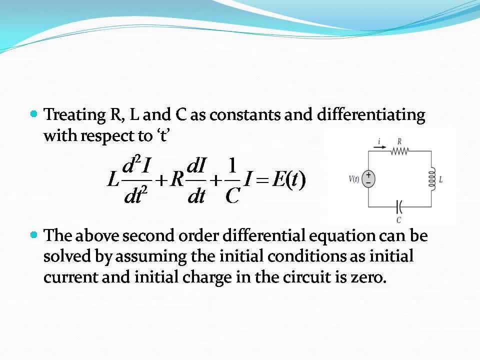 L into di by dt plus 1 by c. q equal to E of t. And now, by differentiating these equations and by treating L, R and C as constants, we get a second order differential equations: L d square, i by dt, d square plus R, di by dt plus 1 by ci equal to de by dt. Here we have replaced dq by. 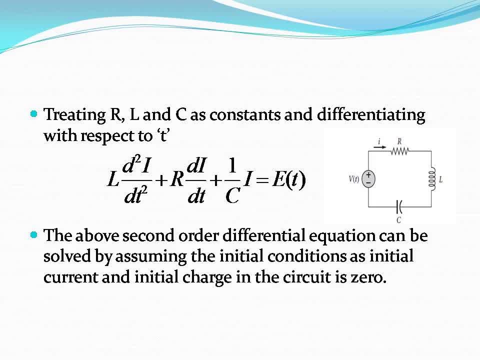 dt equal to i. Now this is the second order differential equations. So by solving the second order differential equations we can find I of t. For that we require the inductance L, the resistance R and the capacitance C. 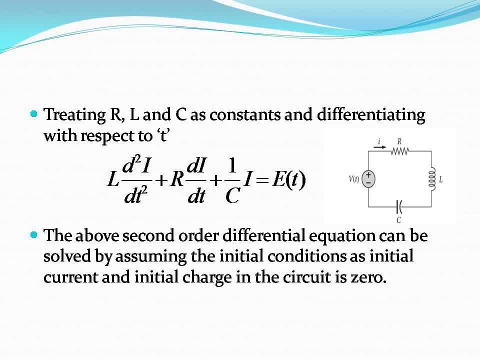 And also we have the initial conditions that the initial current is zero in the circuit and also the initial charge in the capacitor is zero. So with the help of these initial conditions we can solve the differential equations. So we can understand that how. 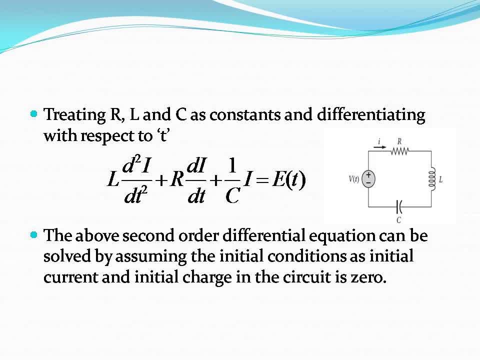 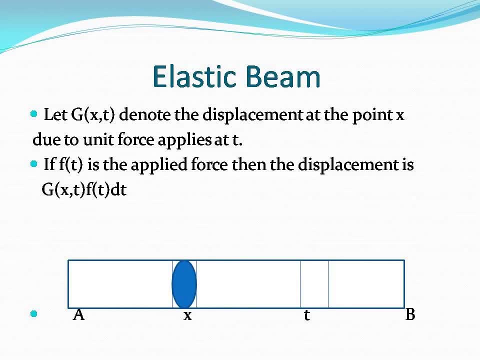 a differential equation helps us to analyze the electrical circuit. So next we are going to see integral equations arising from problem elasticity theory. So here we consider An elastic beam. So elastic beam is capable of expanding due to the elasticity present. 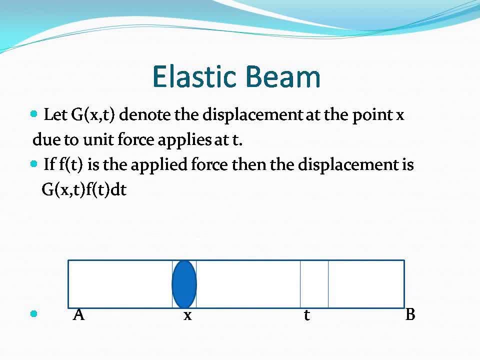 in it. So in this elastic beam we have the endpoints A and B and here if we are applying force at the point T, then due to the elasticity present we have a displacement, x. Now here we have a function, g. So g here is a function due to the elasticity of the object. 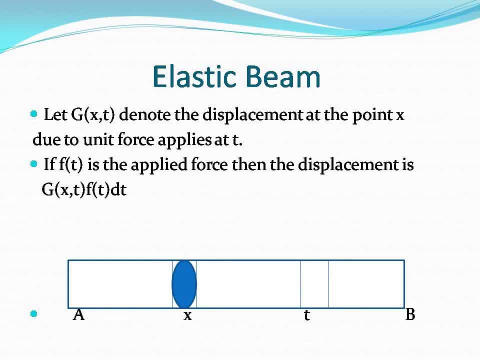 So this g can be found from the equations of the elasticity theory. So g is known, So g is known depending upon the elasticity of each object. So in this elastic beam also we will be able to determined what is g. So now, if we apply a force small, 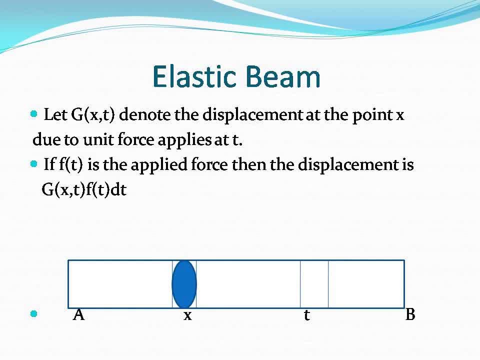 f at the point t, then the displacement at x is determined by g into f, dt. So if you apply one point, then we can find the displacement due to this force along with elasticity. So here the displacement due to the force factor as well as the elasticity present in the beam. So if we apply at one, 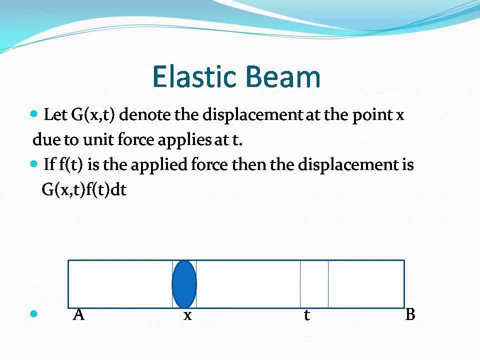 point, the displacement would be g, f, dt. And if we apply at all the points, if we apply at all the points in the beam, then also we can calculate the displacement at a point x. So here we are calculating a displacement at a particular point x due. 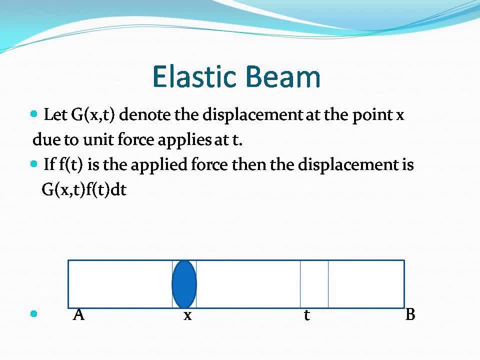 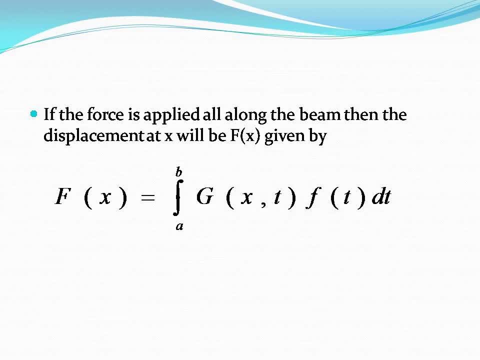 to the force being applied at all the points in the beam. So this is given by. so the force is given by integral a to b, g, f, dt, because we have to take the consideration of the force applied at all the points. 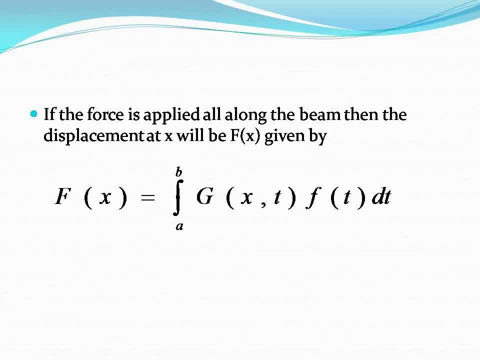 So g is given by being a at all the points and along with the elasticity factor, g multiplied by f, And we take the integral between a to b, we get a displacement at a particular point, x due to the force applied, due to the force applied at all the other points. So 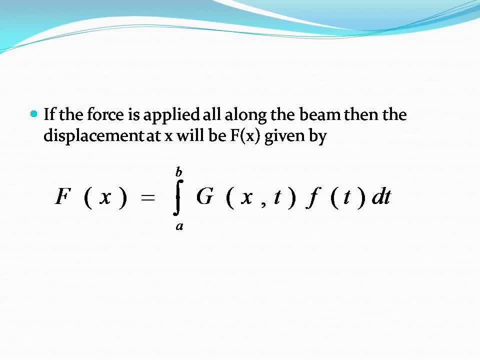 capital, F is given as the integral a to b, g, f, dx. So if you are given small f dt, we can calculate the moments of the displacement. If you have 2 points at the end, this is y. Since y and z are notumbled physically, we soult. 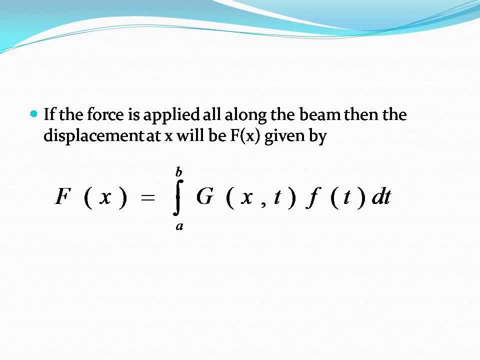 we can calculate capital F directly, But in some situation we will be knowing what is capital F. then the problem is to find what is small f, because we know the effect of the elasticity, and only the effect. we are known and the cost we have to. 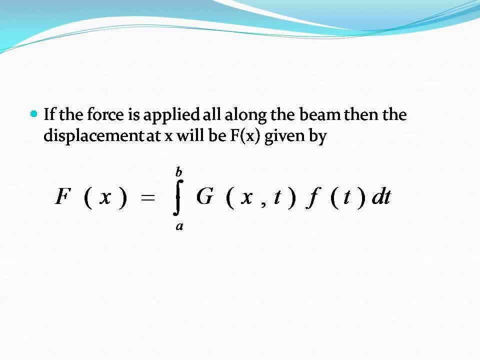 find. So the cost is found by determining small f. So this is called the inverse problem. So this is called the inverse problem is to determine F when capital F is known to find the force distribution which will cause a desired displacement distribution at all the points of the beam. So here the unknown function is small f, where the 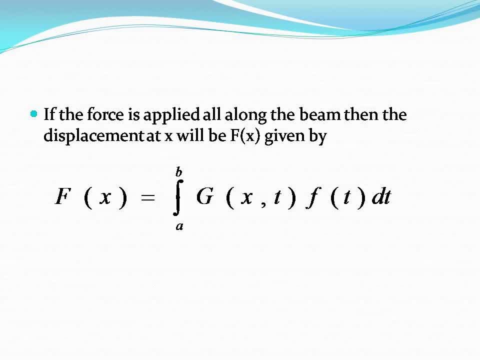 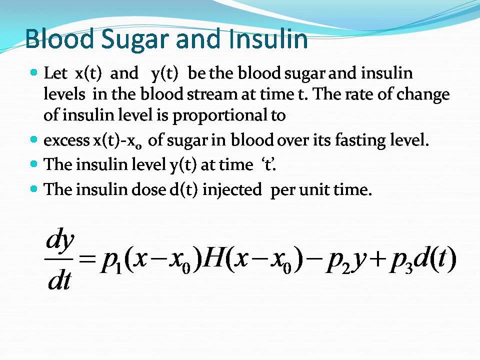 known function is capital F, So this equation is given in terms of the integral equations. So, solving this integral equations, we can find small f, The force applied to the various points in the elastic beam. Here we are going to consider the rate of change of blood sugar and insulin levels in. 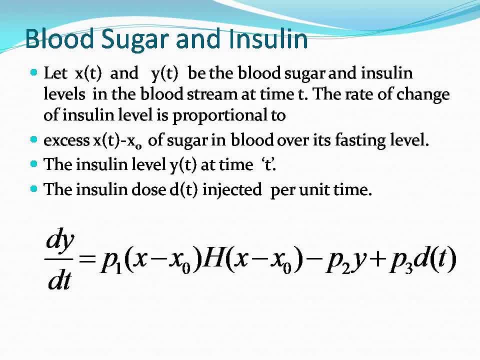 the blood stream at any given time t. Let x and y be the blood sugar and insulin level in the blood stream at time t. and when we analyze the rate of change of insulin level, we are to consider 3 factors, That is, if x0 is the blood sugar level in the fasting. 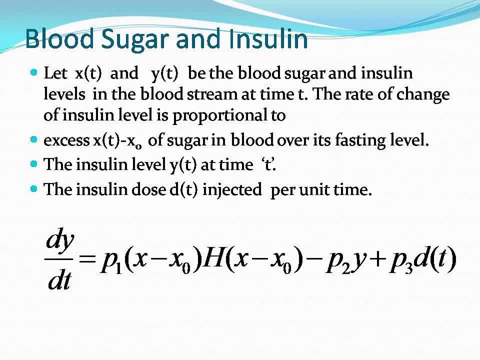 level. if we denote x0 as the blood sugar level in the fasting level, then the rate of change of insulin will be proportional to the xs sugar x of t minus x0 of sugar in blood over its fasting level, because the more the amount of sugar present in the blood 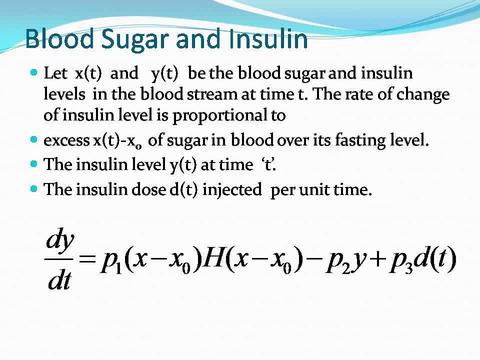 The more insulin it is required to secrete. So and it is also proportional- negatively proportional- to the insulin level Y of T at time T, Because if already some insulin has been secreted, then as time progresses it will be proportional to the amount of insulin level which is secreted at the time T. 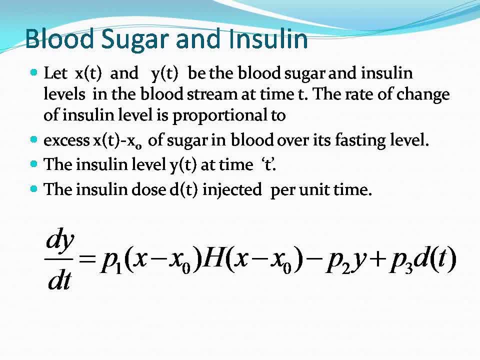 And finally, it is also positively proportional to the amount of insulin which is being injected per unit time. So when we inject insulin in the blood and this insulin will be secreting because of the injection, it will be secreting into the blood at some rate. so that is denoted by D of T. So DY by DT is positively proportional to D of T. 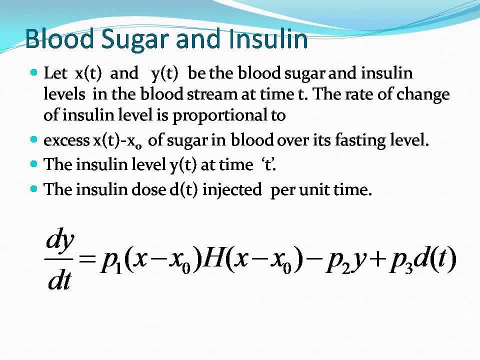 So when you put the proportional constants We have dy by dt equal to p1 of x minus x0, h of x minus x0.. So here h of x minus x0 is a function where we define. h of x minus x0 is equal to 1 when 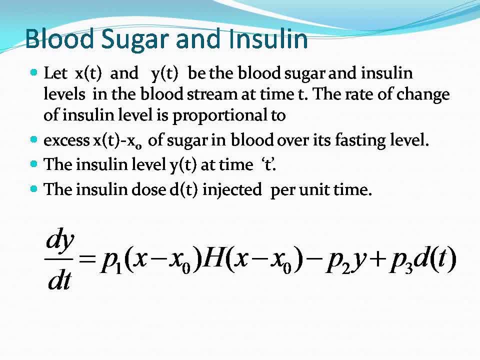 x is greater than x0. H of x minus, that is, if the sugar level is more than the fasting level, then this factor is equal to 1.. So it will be nothing but p1 of x minus x0.. If x is less than or equal to x0, then h of x minus x0 will be equal to 0. 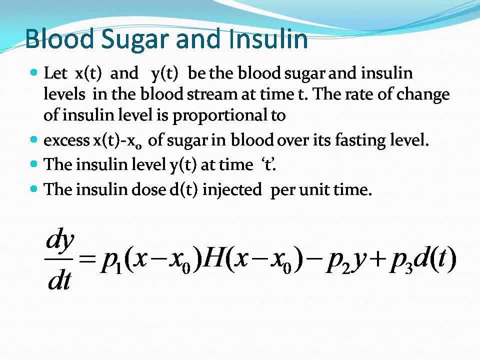 Therefore this factor will not come into consideration. if sugar level is below the fasting level, then it will not come into consideration because there is no incident required, because it is already in a state of low sugar. So dy by dt equal to p1 of x minus x0.. 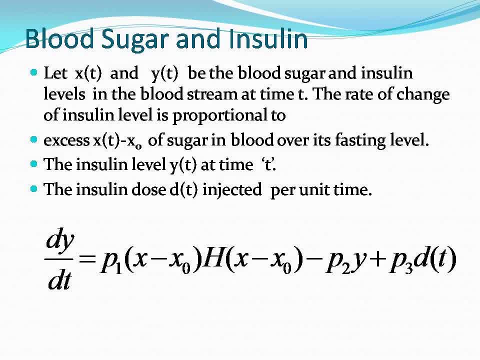 h of x0 is equal to 1.. minus x naught minus p2 yy, because it is negatively proportional to the amount of insulin present at the time t. So it is minus p2 of y, plus p3 into d of t. d of t is the amount of insulin. 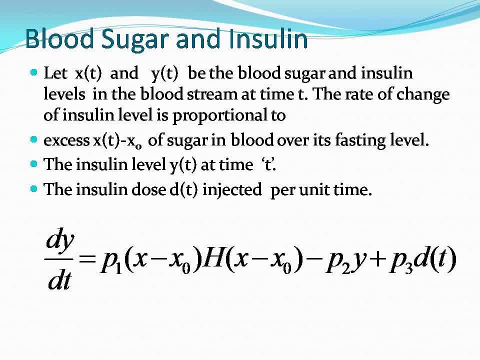 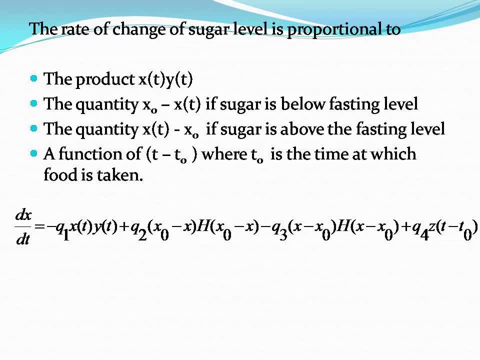 dose injected per unit time. So this is the equation governing the rate of change of insulin level. Now the rate of change of sugar level. rate of change of sugar level is proportional to the product x of t and y of t. It is negatively proportional to the product x of t and y of 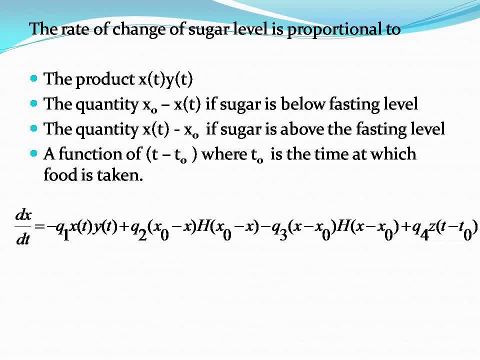 t, because if already, if a sugar level is present at a considerable level, then the sugar need not rise as rapidly. If the sugar is high, then the possibility of sugar rising is low. Only when the sugar is low, the sugar rising possibility is more. Therefore, dx by dt is: 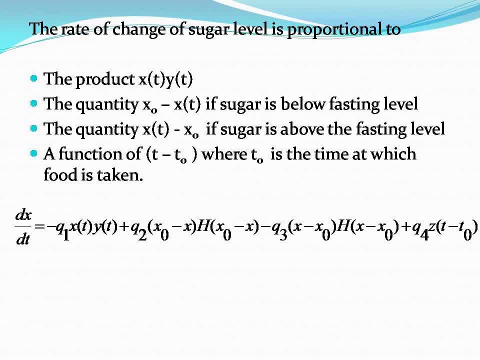 0. Minus q1 of x of t into y of t, And it is. the rate of change of sugar level is also proportional to the quantity x naught minus x of t. if sugar level is below the fasting level. If sugar is below the fasting level, then that means we have low sugar. That means 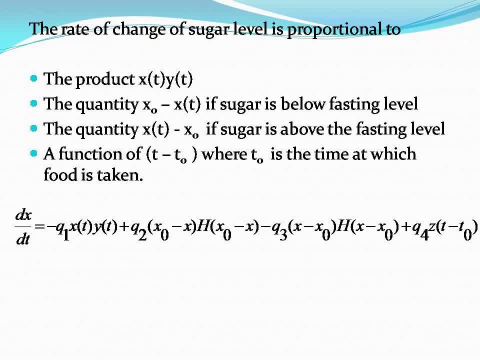 the sugar. it is likely the sugar is going to rise, That is, it is more likely that the sugar is going to rise when the sugar is on a low level. Therefore, it is proportional to x naught minus x of t. So we have the term q2 into x naught minus. 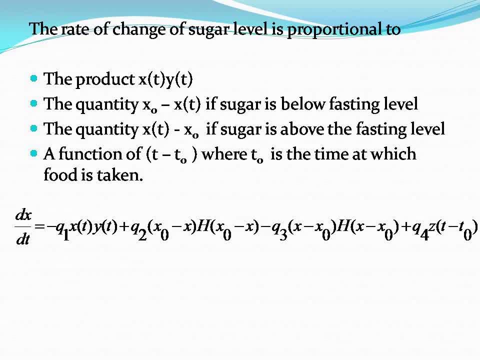 x, But this is only when the sugar level is below the fasting level. Therefore we have a term h of, So it ensures that the product is present there only when the x naught is greater than x, That is, the sugar level is below the fasting. 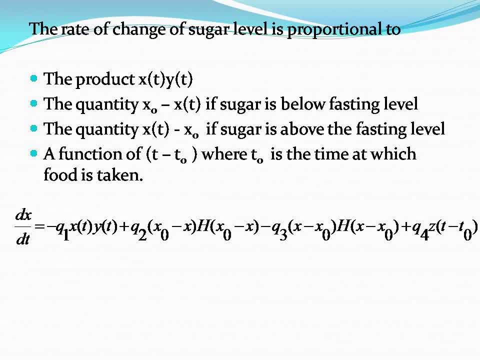 level. If the x naught is less than x, than this whole term will not be there. This q2 will not be there. If x naught is greater than x, then it is either higher in q2 or h of dx. It is not going to increase and decrease in chicken spectrum if this over. 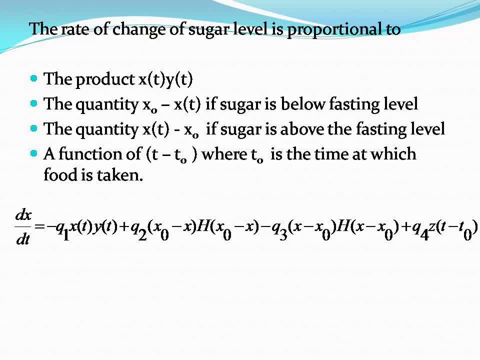 the fasting level is less than x, Then the whole term does not exist, So there is Baronians' A x. then it is just equal to Q 2 of x naught minus A x And the rate of change of sugar. it is also proportional to x? x of t minus x naught if sugar is above the fasting level. 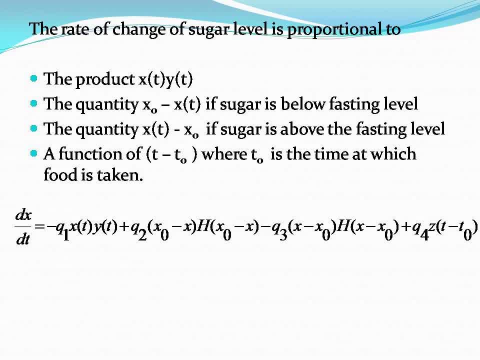 That means if sugar is more, then again the rate of change of sugar level is negatively proportional to the already the amount of sugar present. So we have here again we are, multiplying by h of x minus x naught, to ensure that x is greater than x naught. 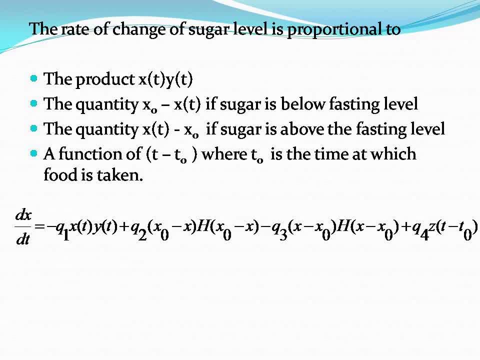 If x is less than x naught this term, the whole term is going to be 0. That is Q 3 of x minus x naught. this term is not required. And finally, the sugar level is also proportional to a function of t minus t naught, where t naught is the time at which the food is taken. 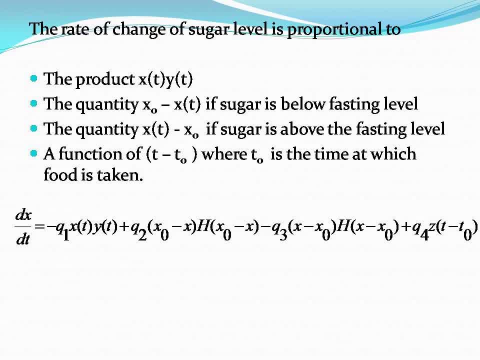 Some function where, say, z z of t minus t naught, where t? naught is the time at which the food is taken, z is the function from which time has proceeded from the food taken last time. So t minus t naught denote the amount of time that has passed after taking the food. 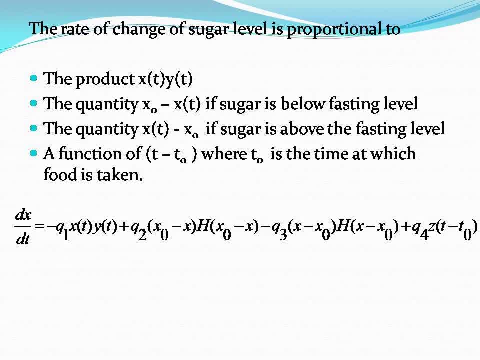 So it is also proportional to z of t minus t naught. So we have the differential equation concerning the rate of change of sugar level. So here you can see that d x by d t and d y by d t are both. 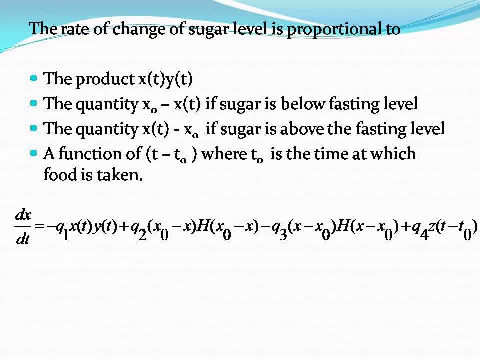 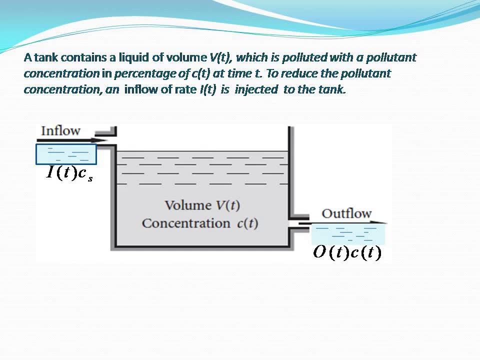 They form a simultaneous, non-linear differential equations And these are the equations which governs the rate of change of sugar level and insulin level. Now we consider a liquid tank containing a volume v naught. So initially this tank contains a volume of liquid v naught, with pollution concentration v naught. So initially this: 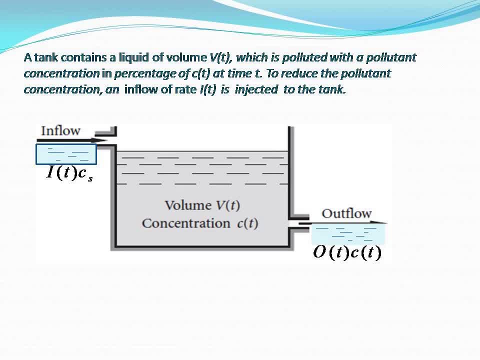 tank contains a volume of liquid v naught with pollution concentration c naught. So initially this tank contains a volume of liquid v naught with pollution concentration c naught. So initially this tank contains a volume of liquid v naught with pollution concentration. 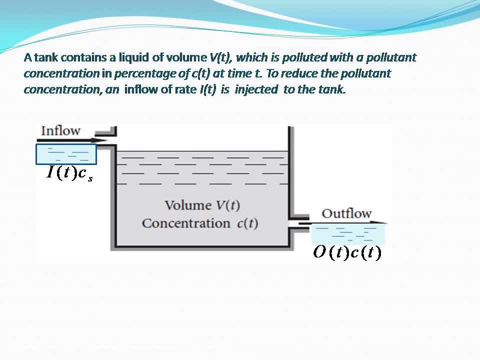 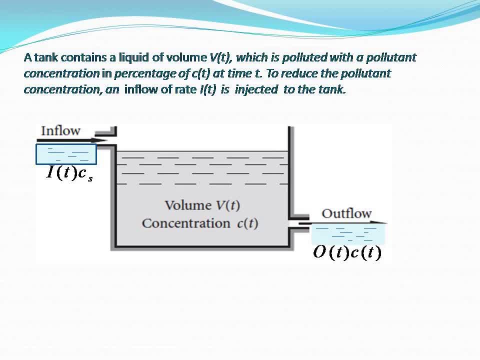 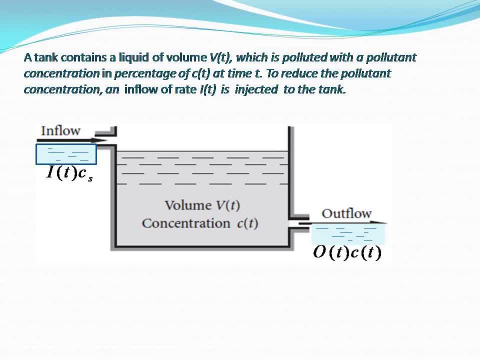 So initially this tank contains a volume of liquid, v naught with pollution concentration, c naught pollution concentration- an inflow I is given into the tank, So the inflow is injected to the tank to reduce the pollution concentration. So as the inflow is injected to the tank, we also have the outflow at any given point. 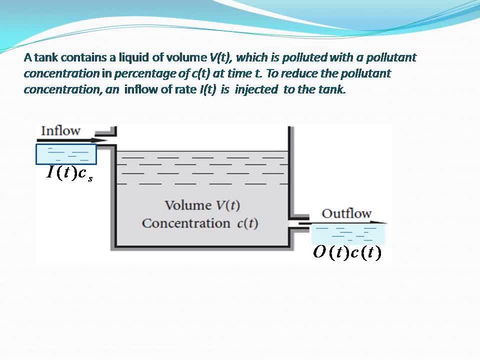 of time, the outflow is given by O, So the rate of inflow is given by I and the rate of outflow is given by O, So constantly, at any given point of time, this inflow is outflow is happening and, as 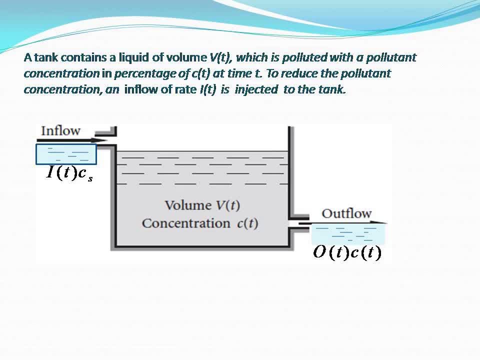 time proceeds. because of this inflow the pollution concentration changes. So this pollution concentration changes Despite to time t. so the rate of change of this pollution concentration is given by the derivative of C. So the derivative of C with respect to time t gives the rate of change of pollution concentration. 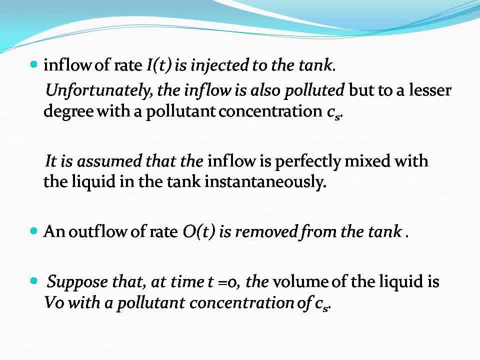 So these are the terminologies. The I is injected to the tank, but unfortunately, the inflow is also polluted, Let's believe, With the concentration CS. The inflow is also polluted with the concentration CS. So, along with the inflow, though. the inflow is given to purify the tank, but it may also contain a pollution concentration, a minimum pollution concentration. 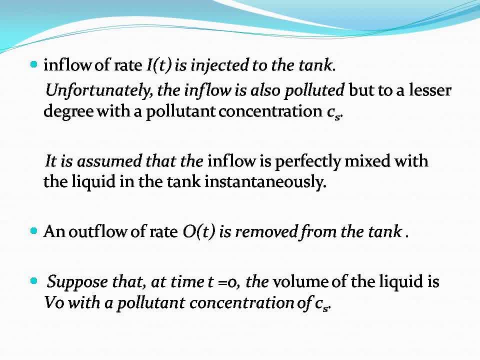 So not as much as in the water tank, but a minimum pollution concentration which will be available in any liquid. So that is given by CS. So this inflow is perfectly mixed with the liquid in the tank instantaneously. So continuously this inflow is mixed with the liquid and continuously the outflow of rate O of T is removed from the tank. 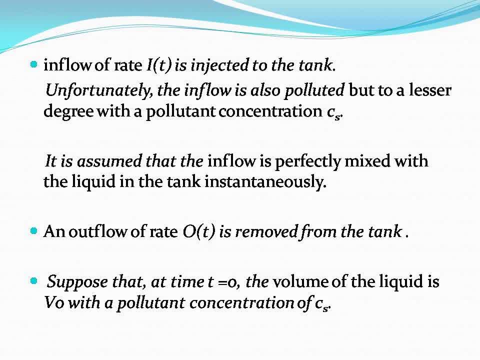 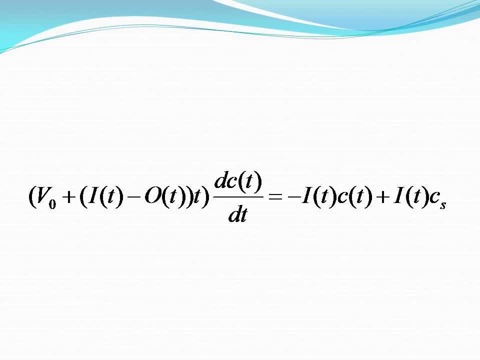 Suppose, at time T equal to zero, The volume of the liquid is V0, with the pollution concentration of C0. Then we can try to formulate the equation which governs this process, starting from time T equal to zero and at any given point of time, the rate of inflow is given by I of T and the rate of outflow is given by O of T. 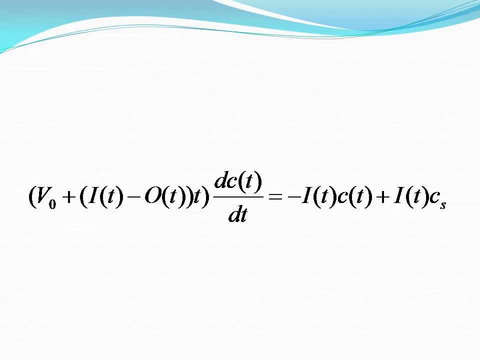 So, since DC of T by DT is the rate of change of pollution concentration And V0 is the initial liquid in the tank at time, T equal to zero. So when we take the difference between the rate of inflow and the rate of outflow, we get the rate of change of the water level present inside the tank. 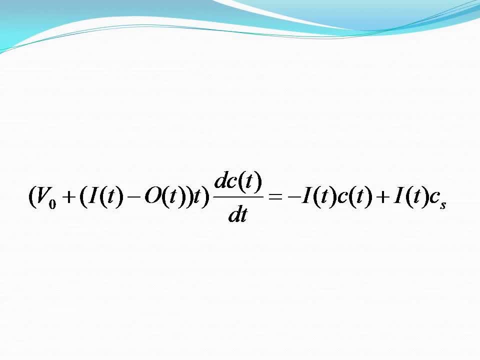 And multiplied with T, we were able to get the total volume of the liquid that is present in the tank. And when we multiply it with the rate of change of the liquid, change of the pollution concentration that should be equal to it should be negatively. 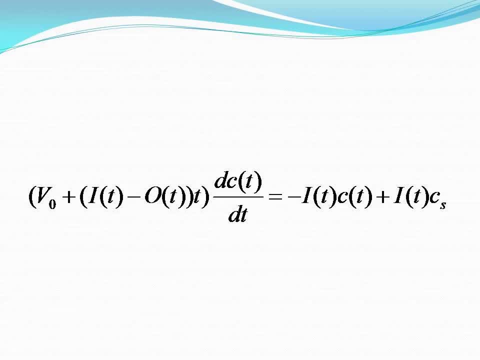 proportional to the inflow, the rate of inflow multiplied by the pollution concentration in that tank. Now the C also changes with respect to time, Because C changes because of the inflow. Therefore this left hand side is negatively proportional to I into C. 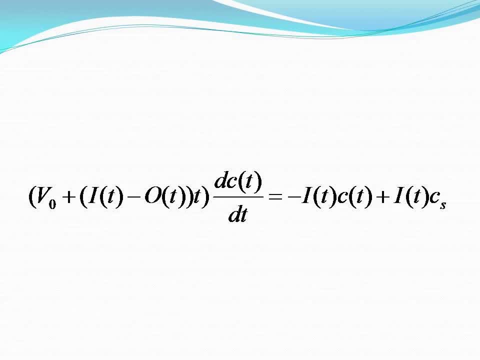 Therefore we have a negative sign, And if the inflow does not have any pollution concentration, then this term is enough. That is minus. on the right hand side we can have just minus I into C, But here the inflow is also polluted with a minimum pollution. 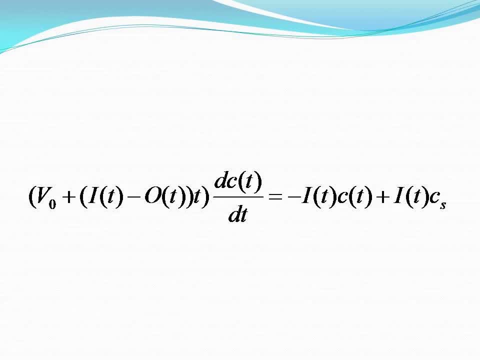 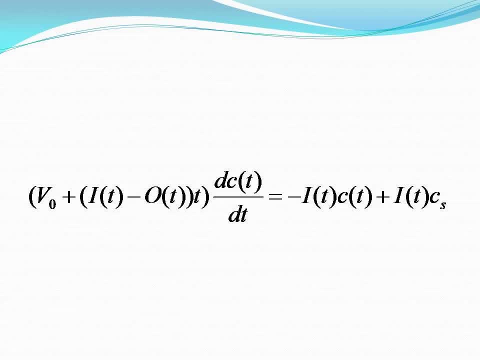 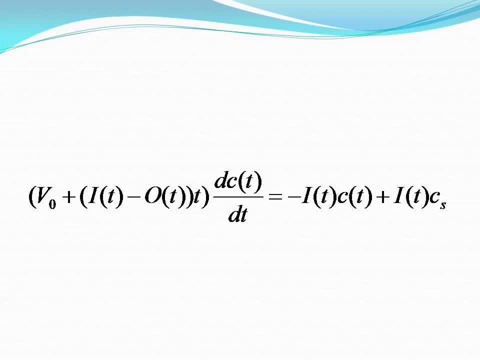 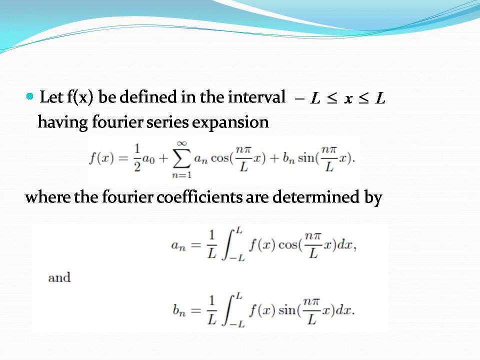 the V0 is a constant And therefore this is a first order differential equation governing the inflow and the outflow process in the tank while purifying the tank from the pollution concentration. Now we are going to discuss the application in recognizing the signal. 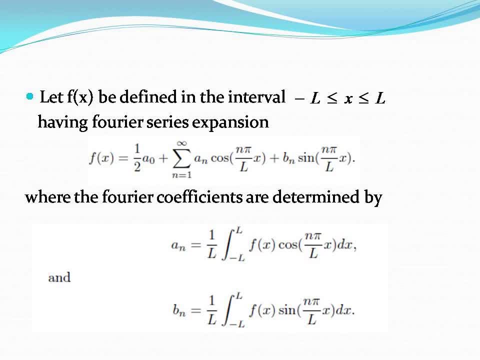 and processing it in the field of remote sensing. For this we consider the Fourier series, expansion. because many signals in the phenomena of remote sensing, the signals are identified with sinusoidal wave and cosine waves, So often the signals are expected to have wavelength that are similar to the sine and cosine. 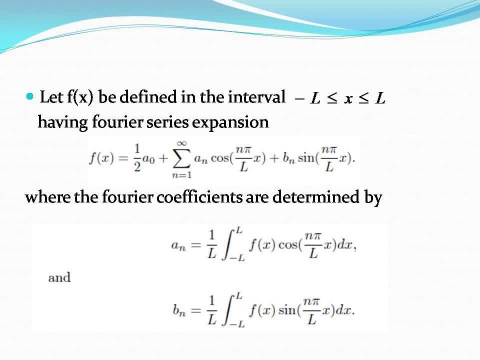 waves. So here we assume that f of x has a Fourier series expansion. that is, f of x equal to a naught by 2 plus summation n equal to 1 to infinity a n, cos n pi x by l plus b, n sine n pi x by l in the interval minus l to l, If l equal to pi. 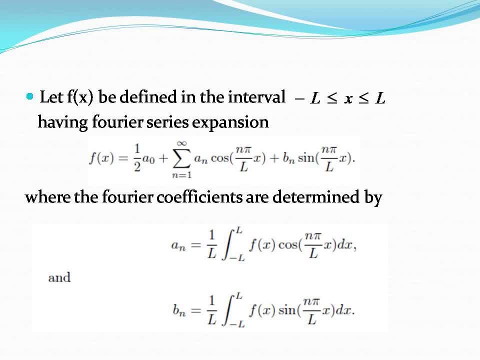 then it will become a normalized Fourier series. expansions, And we know the Fourier series can be determined by these formulas: a? n equal to 1 by l integral minus m to the f of x cos n pi x by l dx. and b? n equal to 1 by integral minus l to the f of x sine pi n pi x by l dx. So if 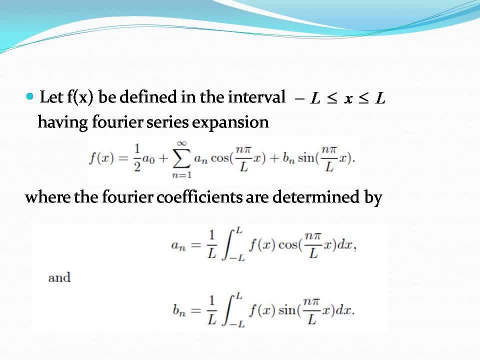 you know all the coefficients, we can determine f of x. So this Fourier series expansion helps us in applications in various ways. One thing is if you know the wave, if you are able to determine the wave fully, then we can change the wave into digitalized wave. 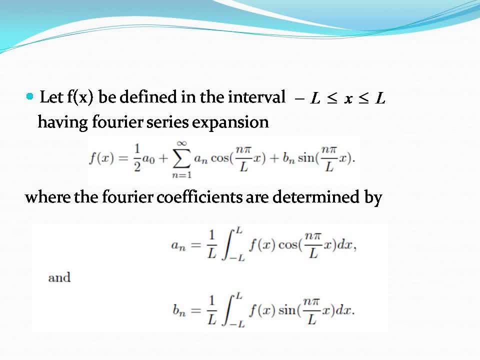 So instead of having the whole wave, we can just have this coefficient, a, n and b n, So that will convert the waveform to digitalized form. So that is one of the concepts used in digitalizing the wave format into the other format, like mp3 and other digitalized format. 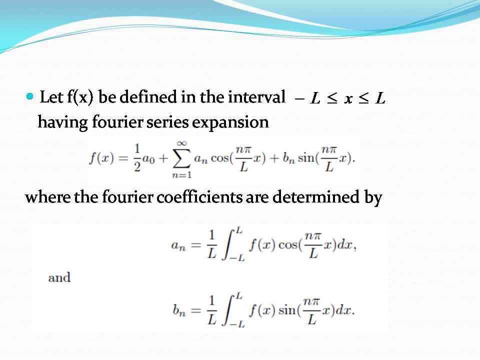 where the waveform is converted into these coefficients a? n and b? n. And another problem is if you want to find the f of x. if you want to find the f of x, then we need to find a? n's and b? n's. So if we are able to find a? n's and b? n's, then we can find f of x. 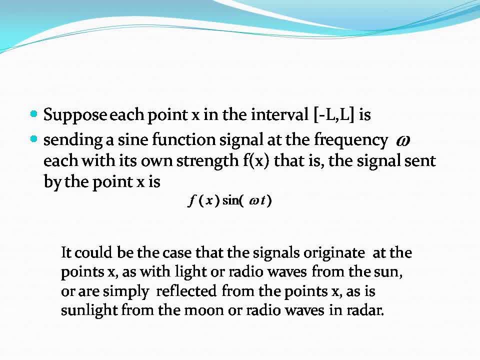 Suppose each point x in the interval minus l to the l is sending a sine function signal at the frequency omega. So if the frequency is high, if the frequency suppose sine 2 is more frequent than sine x, So if you are not able to determine the waveform in the whole, 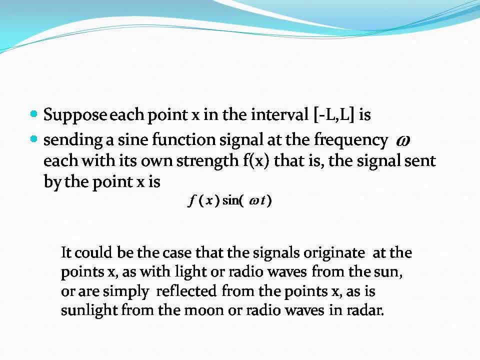 interval, but if you are able to determine at some points in the interval minus l to l which is sending a sine, because you do not know at which point the signal is being received. So if it sends a sine function signal at the frequency omega, each with its own strength. 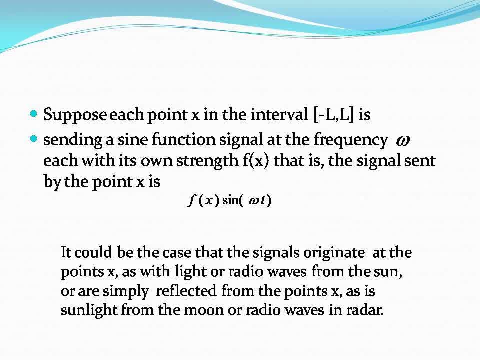 f of x. that is the signal sent by the point. x is f of x into sine omega. So if you are able to find the f of x into sine omega t, So here we are able to determine at the point, using the strength of the signal, as f of x into sine omega t, And here it could be the 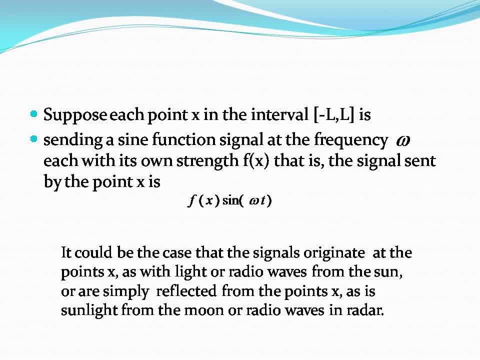 case that the signals originate at the point x, as with the light or radio waves from the sun, or it is being reflected from the point x, as is reflected from moon or radio waves in radar. So if you are able to get more points, if you are able to get more points, that means 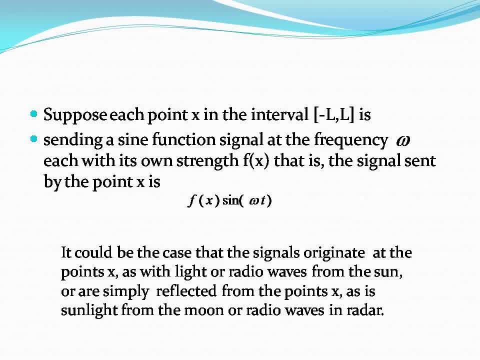 we are able to get points, the terms in the Fourier series, expansion. So the more number of signals we receive, the more accurately we will be able to determine the waveform. So where this is used, This is used in the remote sensing to determine the nature of